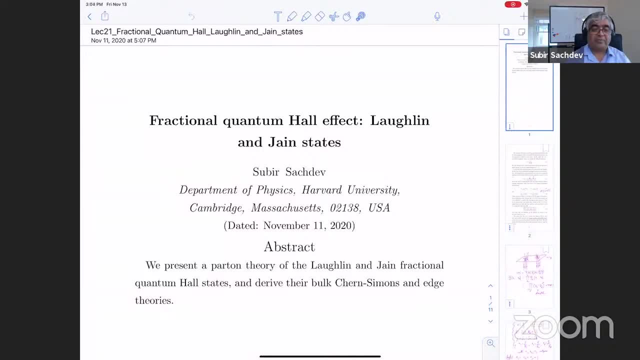 Okay, Okay. So today we're going to continue and probably finish Our discussion of the famous fractional quantum Hall states. So the reason we can be so quick is we've developed all this technology of Chen-Simons gauge theories and fractionalization. 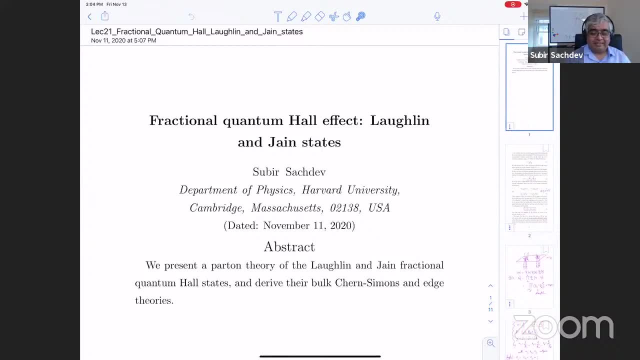 And when we just apply those tools to electrons in a strong magnetic field, we can just reproduce a whole bunch of results. that took the community many years to straighten out. Okay, so any questions? Someone had a question? No, I guess not. 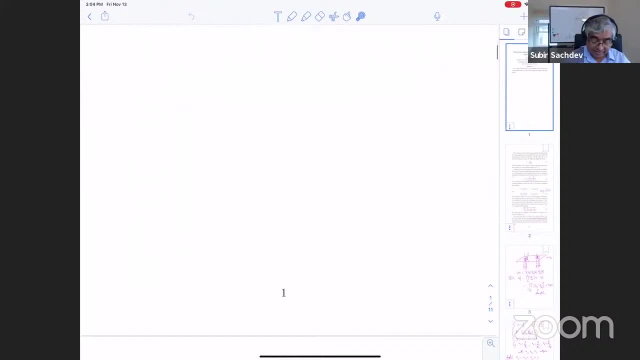 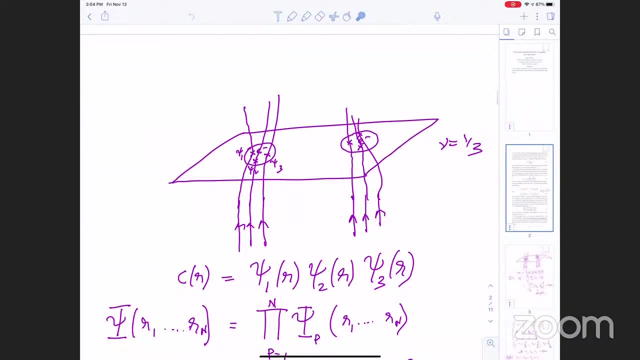 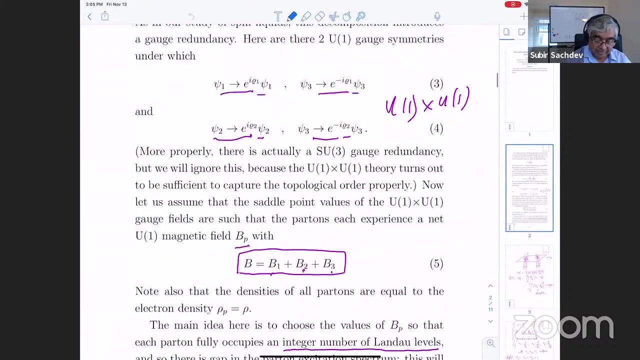 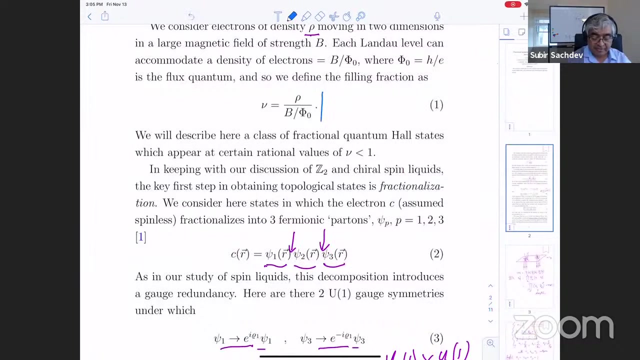 All right. So what we're considering here is electrons in a very strong magnetic field moving in a plane, And the basic quantity that measures the strength of the magnetic field is the filling fraction, which is basically mu. right here, it's the ratio of the density to the magnetic field in units of the flux quantum. 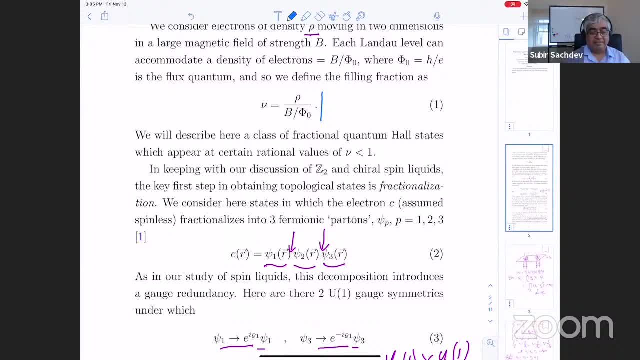 So we just use the flux quantum to measure the field And that gives the B. B just becomes a measure of density And we can talk about B as measuring the number of flux quantum per unit area, just as rho measures the number of particles per unit area. 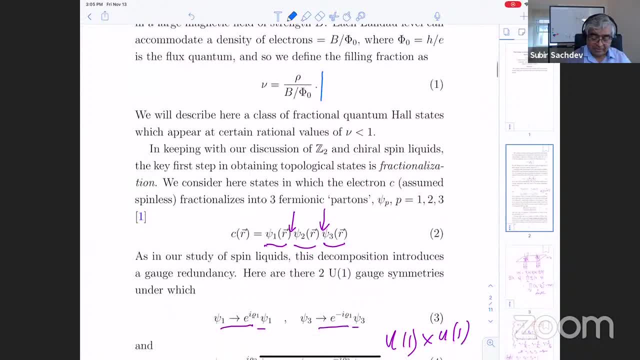 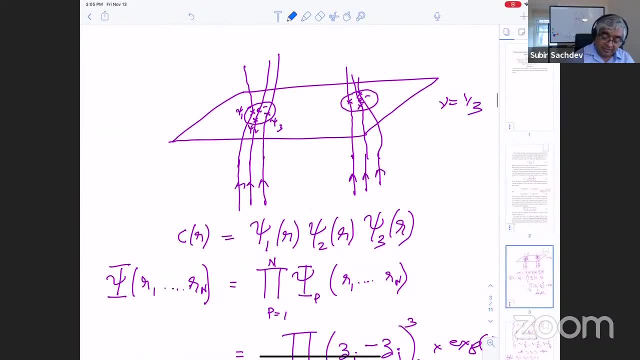 So in a fully filled Landau level of three electrons, the number of electrons equals the number of flux quanta. So if you consider the most famous fractal quantum Hall state, which is some gap state of matter obtained at filling fraction, mu equals one third. 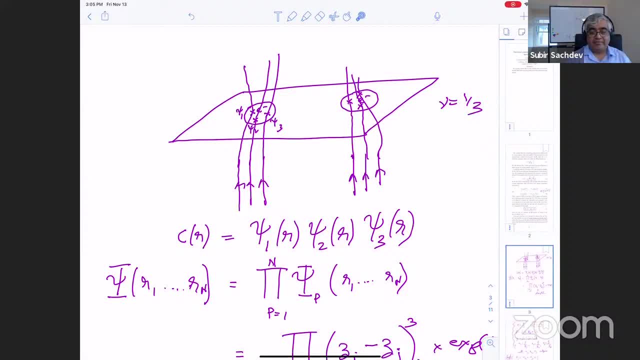 then you have one electron for every three flux quanta, as illustrated in this picture, And so that means that the lowest Landau level is only one third full if you just use single particle states, So naively you would think you know if you have all these states. 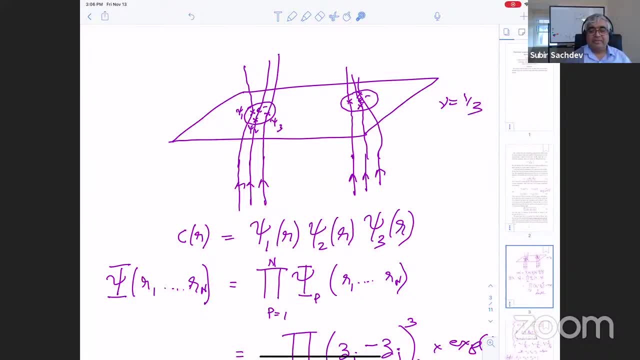 zero energy states in the lowest Landau level, only one third of them are full, So there seems to be a huge degeneracy where these particles can occupy. you know, N choose N over three possible states, which is a very large number. 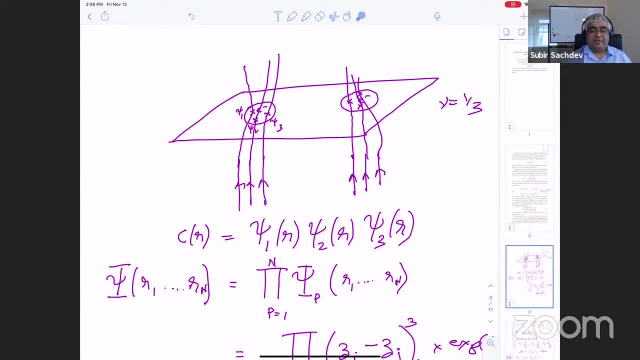 N is the number of states in the Landau level. So you might expect you have lots of low energy excitations. you get some some rather complicated state or you might get some broken symmetry or solids, which is what people expected. 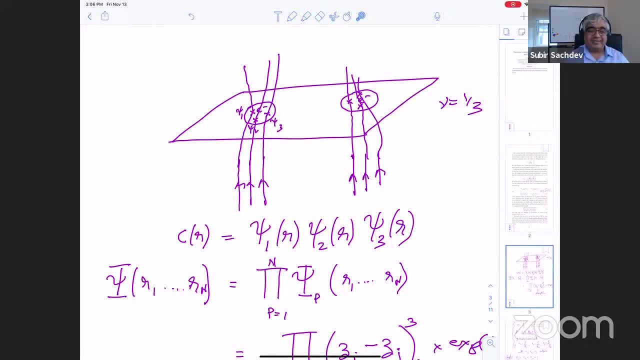 But amazingly, what you get is a state with a gap and it's almost a unique state and has very few low energy, essentially loads at low energy excitations, And that's the, the norm, the Laughlin state, And we understand the state. 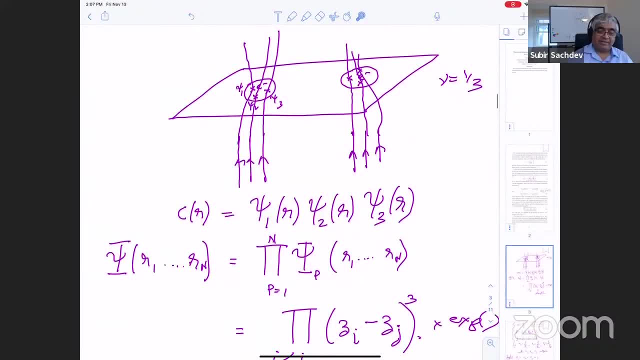 the way I present it is by using our favorite trick of fractionalization, And we think of the fractionalization here as taking the electron operator, ignoring spin, in terms of three protons. And once you have the three protons, then roughly speaking, 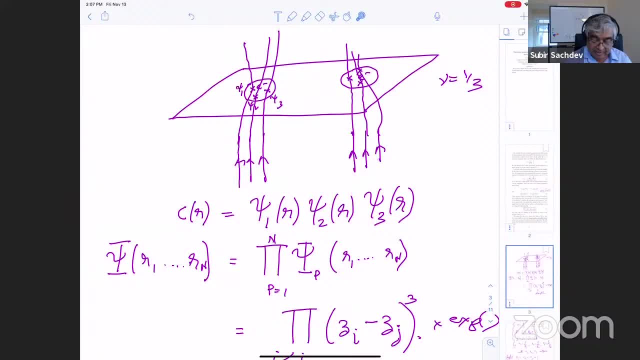 you can imagine that the external magnetic field gets split into three pieces, where one flux quantum attaches to one of the protons. Okay, so now, of course, the key thing here. these protons are not independent particles. Their coordinates are the same as the coordinates of the electron. 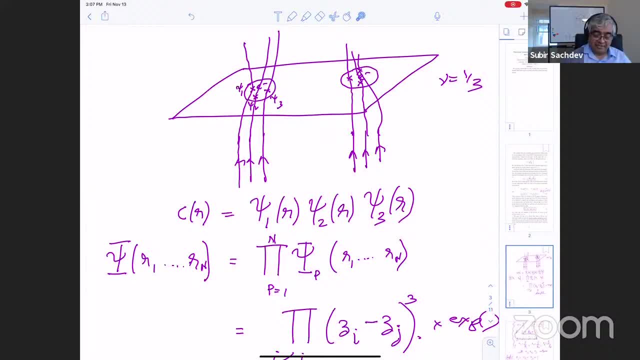 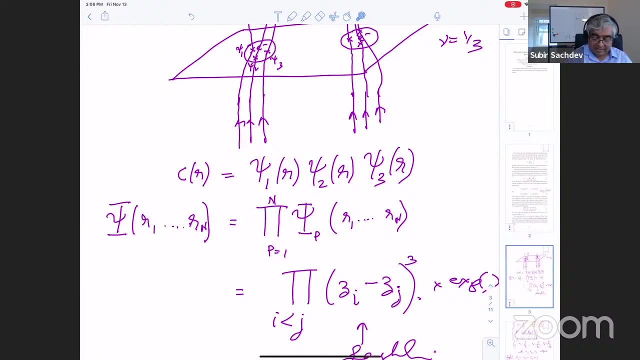 But momentarily. let's imagine they're independent particles each moving in their own magnetic field, And just to conserve total magnetic field, each of them has exactly one flux quantum. So the wave function of the electrons will be just a product of the wave function of the protons. 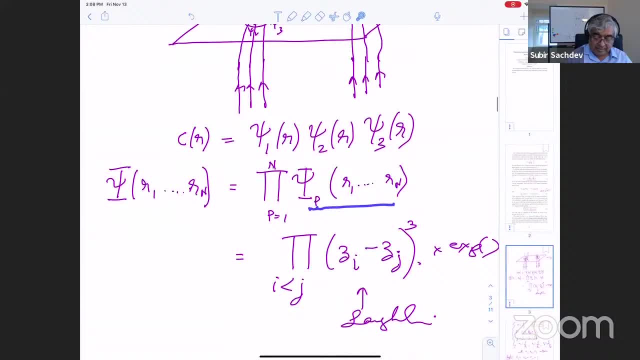 And each proton has this wave function which is a particle in the lowest Landau level. So this one proton wave function, then psi, p, so for example, psi one is just the lowest Landau level state which we saw a while back. 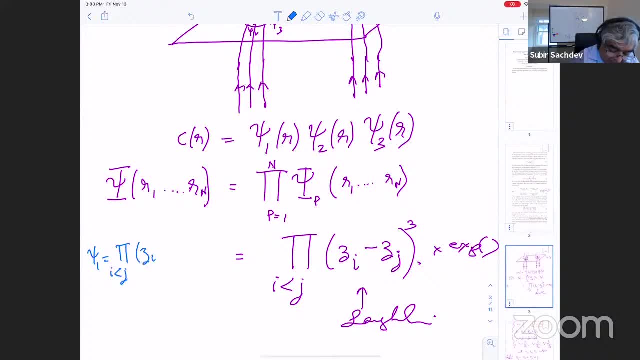 apart from some exponential factors, was just z i minus z j. So you just take the product of that, So you get z i minus z j cubed from the three protons, and that is the famous Laughlin state. So that's kind of a cute construction. 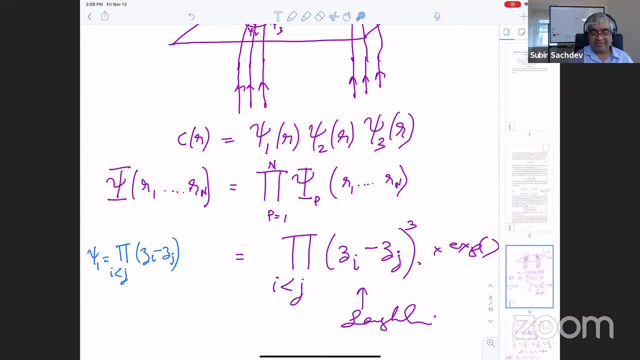 Laughlin just pulled out his wave function just by some guesswork, brilliant guesswork, And this is just another way of getting it, but it has the power of allowing us to also say a lot more, because it directly leads to the Chen-Simons gauge theory. 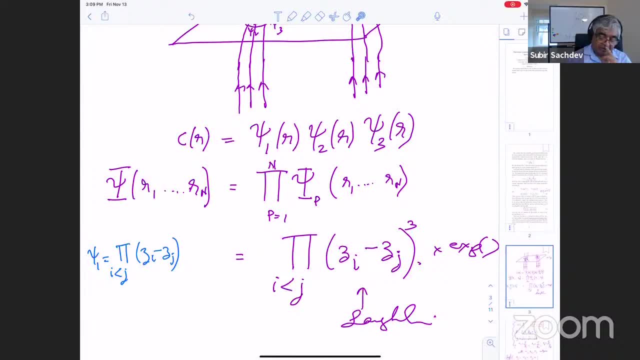 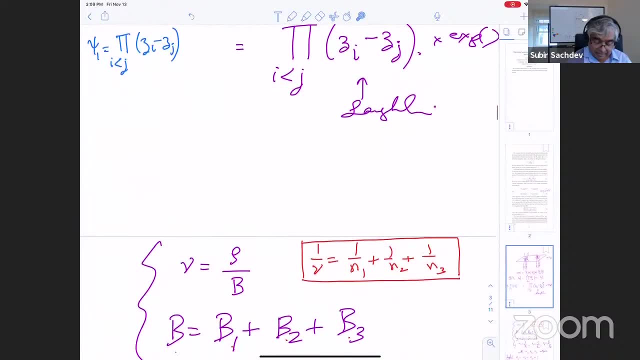 and the T of the edge states and all of that, all of those properties also follow from this part-on approach, which is what I'm going to show you today. All right, In general, the more general way of saying the part-on approach. 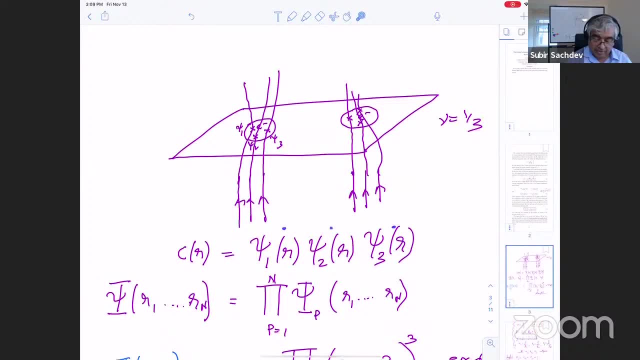 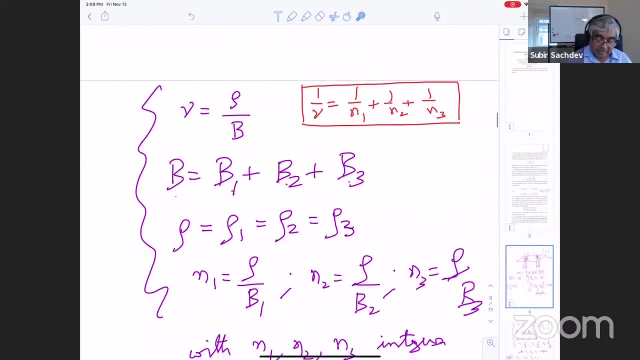 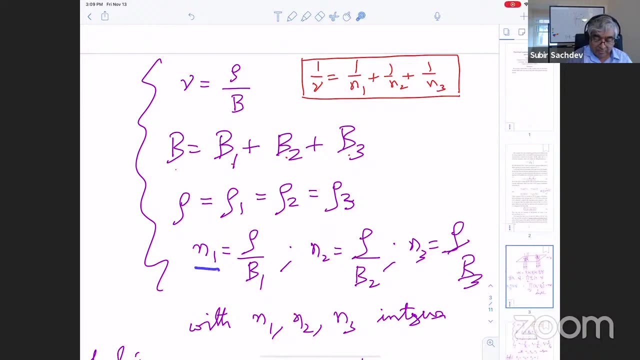 is that each one of the part-ons should occupy an integer number of Landau levels. So let's imagine that the pth part-on occupies np. Landau levels little n. So the first part-on has Landau levels n1.. The second part-on has Landau levels n2.. 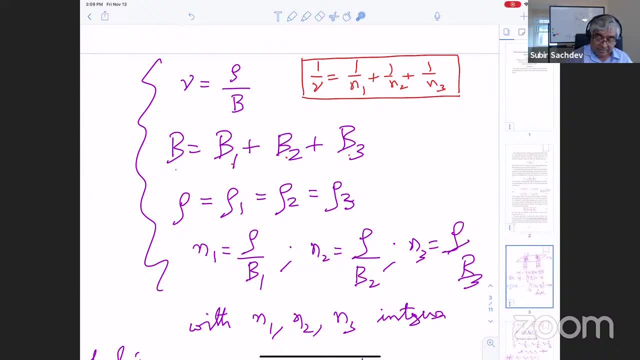 The third one has Landau levels n3. And this is, of course, related to the ratio of the density to the magnetic field that each of them experiences. Okay, so n1,, n2, and n3 are integers, And 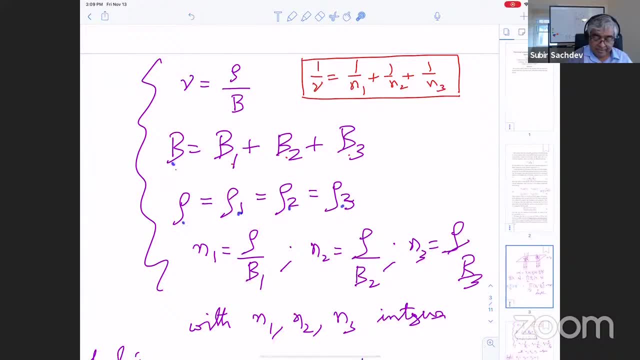 Okay, So the density of the three have to be equal and the b field has to be the sum of the fields. And if you play with these equations, you get this equation for the filling fraction nu of the electrons, where n1,, n2, and n3 are integers. 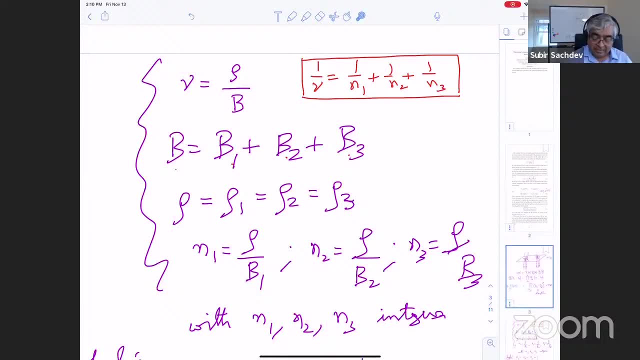 So for these integers, we have a simple construction of some gap state, which is, you know, quite remarkable, And the states we'll talk about are all of this type, where two of the integers are one and the third is one for the Laughlin state. 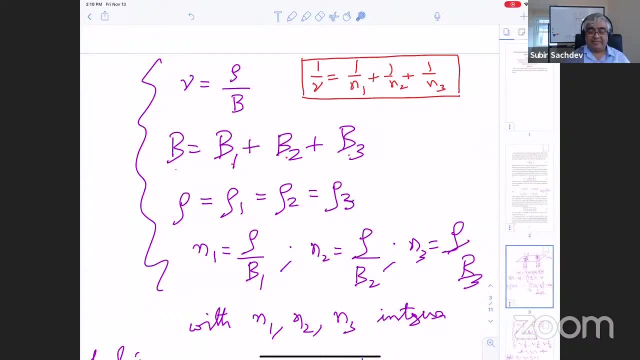 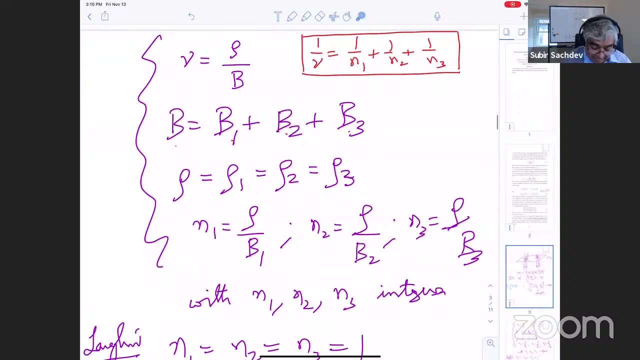 and greater than one for the Jain states, And those pretty much by and large, with very few exceptions, exhaust the set of states that are seen So Okay. So that's why we're focusing on them, and it's quite remarkable how well this works. 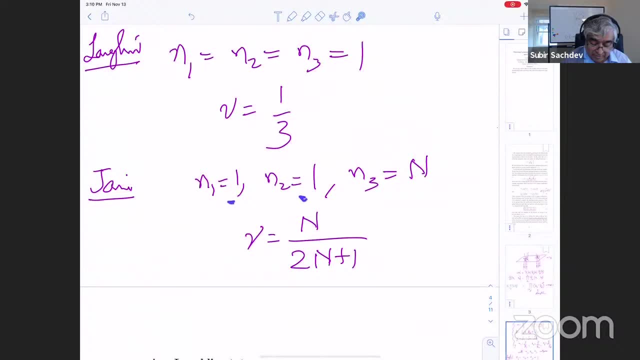 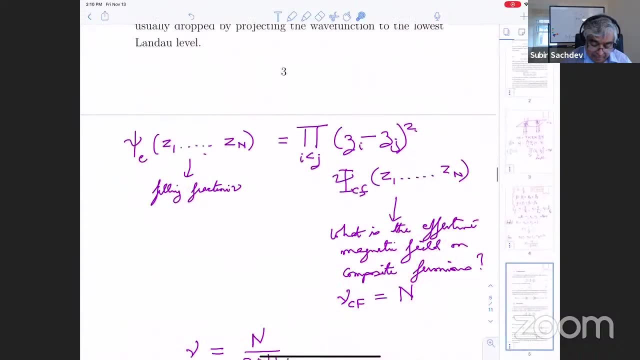 Okay, Yeah, so the JN case corresponds to n1 equals 1, n2 equals 1, n3 equals n, and nu is 2n over 2 plus 2n, n plus 1.. Okay, So actually let me say a bit more. 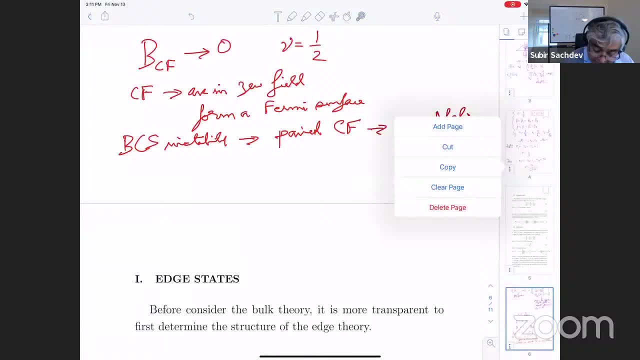 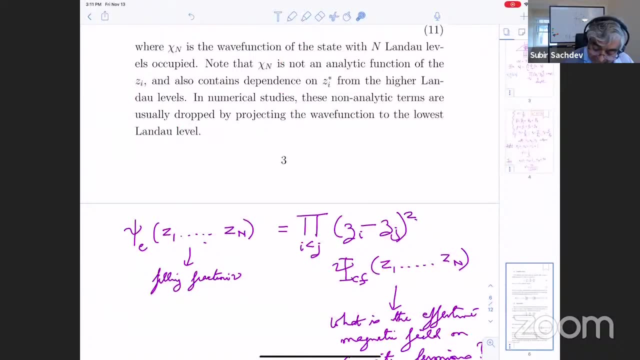 about the gauge theory structure of it, and then we'll extend that to the edge states. I mean, I've said it in the notes, but rather tersely. Maybe I should be a bit more explicit. Go on the page. Sometimes it doesn't appear. 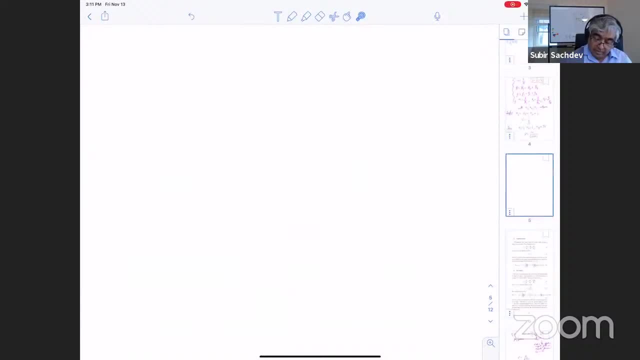 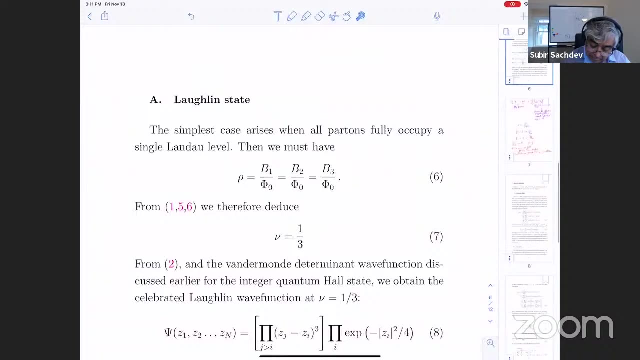 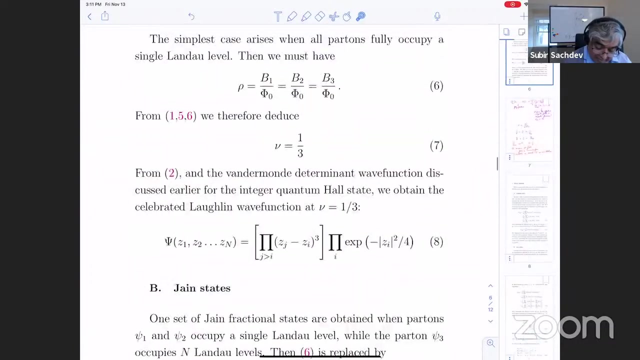 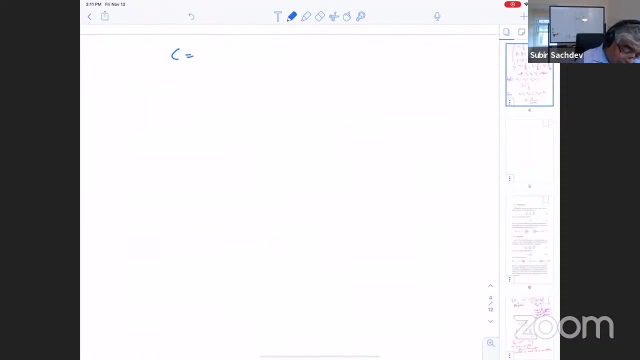 There, it is Okay. Any questions so far? Yeah, I guess I haven't even bothered to say what the gauge fields look like, Just say it in words. All right, So you have this decomposition. C equals psi 1, psi 2, psi 3.. 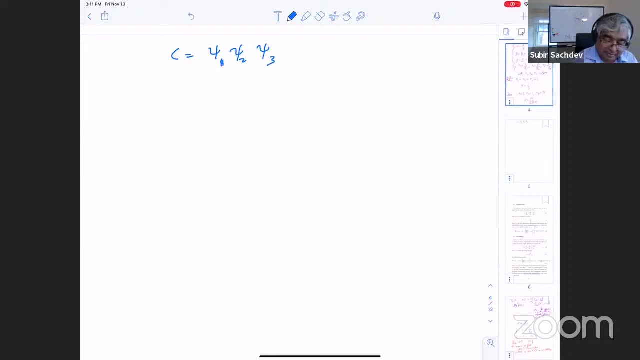 So this means there are two gauge fields under which the theory is invariant and we'll have to account for these two gauge fields. Then psi 1 goes to psi 1 times e to the i rho 1, and psi 3 goes to psi 3 times e to the minus i rho 1.. 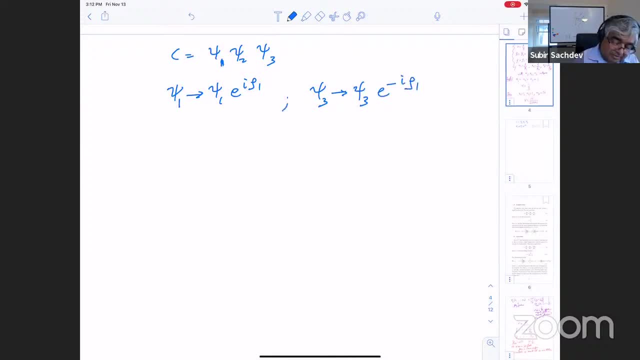 So the psi 1 and psi 3 have opposite charges under the gauge field. We'll call it this is a u1 sub 1 gauge field. And then there's another gauge field where psi 2, which is a u1 sub 1 gauge field. 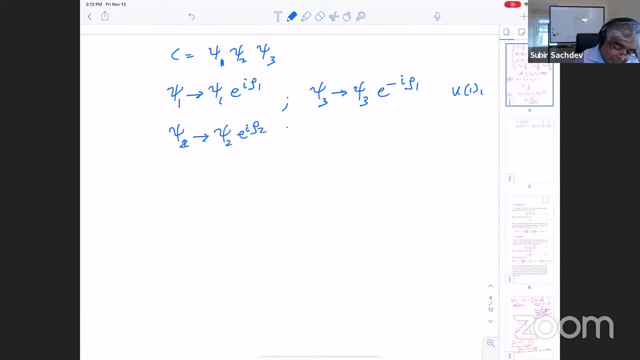 goes to psi 2, e to the i rho 2.. And psi 3 goes to psi 3, e to the minus i rho 3.. And this is another gauge field, rho 2.. Called u1, sub 2, just to distinguish it. 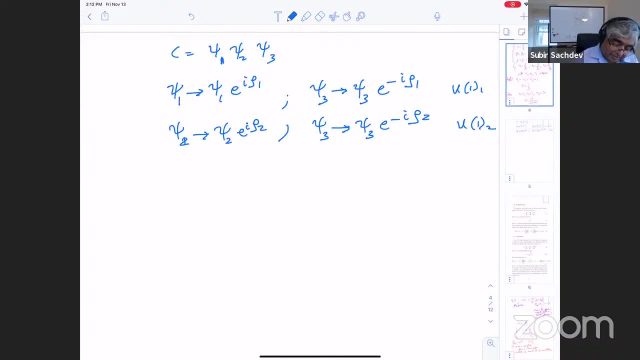 So now, if we write down some action for psi 1, let's write down just the kinetic energies. We also have the kinetic energies, the external magnetic field which, let's us assume, acts on psi 1.. So then I will have on psi 1,. 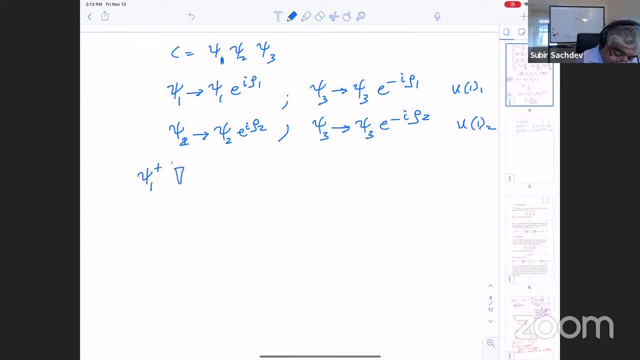 I'll have psi 1, dagger grad minus the external field a, and then an internal field with respect to the first one, So that'll be minus. let's call it i a1.. So i1.. And then for psi 2,. 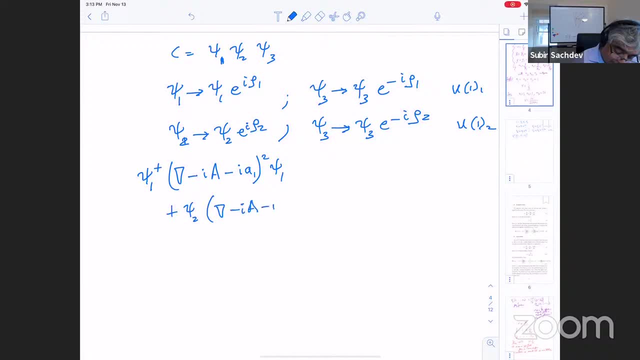 you'll have the same thing: grad minus i, i a, minus i a2, psi 2.. And for and for psi 3, you'll have grad minus i- a, but now it's got both of these gauge fields acting. 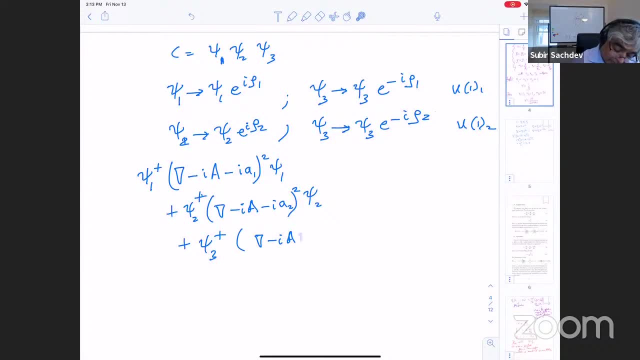 but with the opposite sign. So that'll be plus i a. Okay, so this is our gauge theory. We have two internal u1 gauge fields and also an external gauge field. Now the key here. oh, and I'm sorry, I made a mistake. 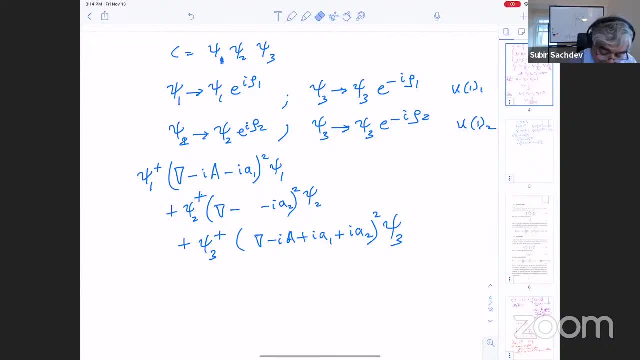 There is no external gauge field acting on the others. It only acts on one of them. Okay, Right, Okay. So now what we want is for the. let's see, I hope I get this right. This is two thirds. 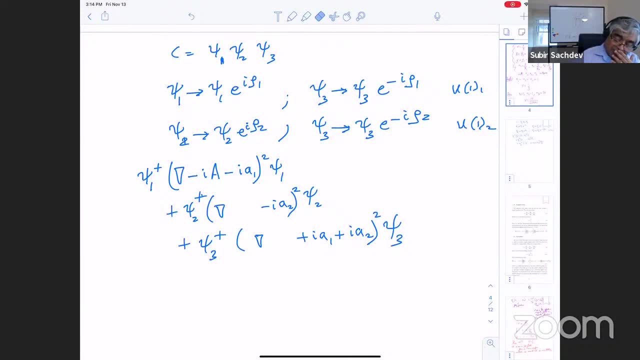 Yeah, Okay, I hope I will. I'm suddenly very confused. Let's see That's row one. That's correct, That's right, Okay. One minus two thirds minus two thirds, Okay. So Let's do it over. 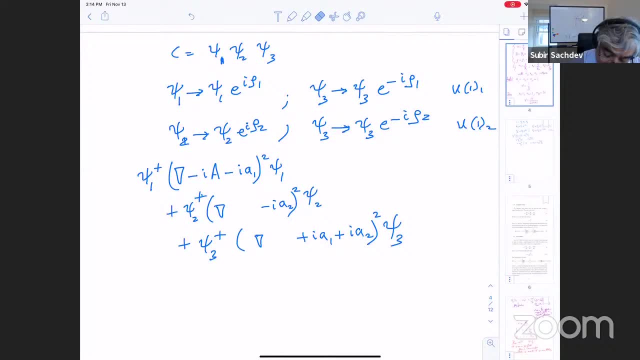 Let's see. So I think this is going to be it's going to be two thirds, So this is going to be two thirds, Let's see. So, let's see How many times did I do it right? Three times. 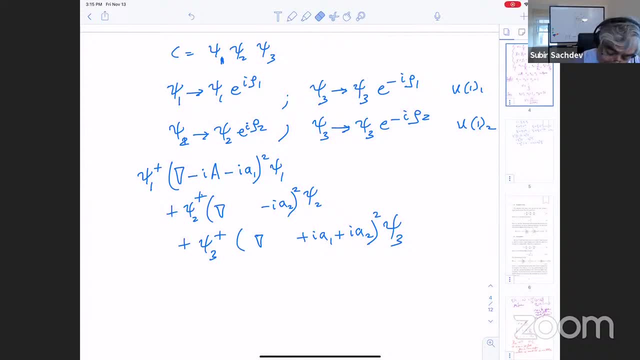 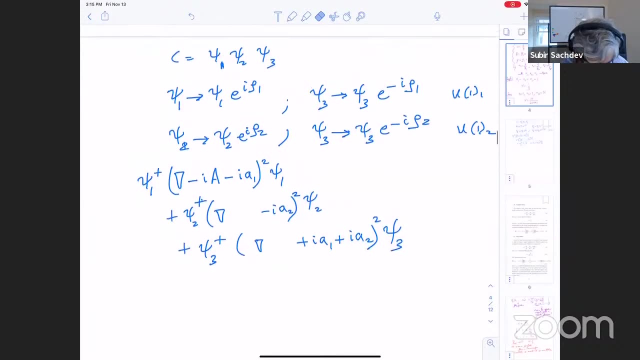 So what is the in the? oh, I'm making a mistake somewhere. What mistake did I make? Oh, I don't know. Okay, Okay, So the I'm going to put the let me, let me. 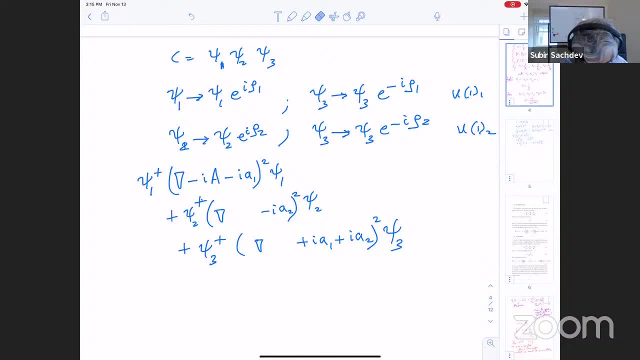 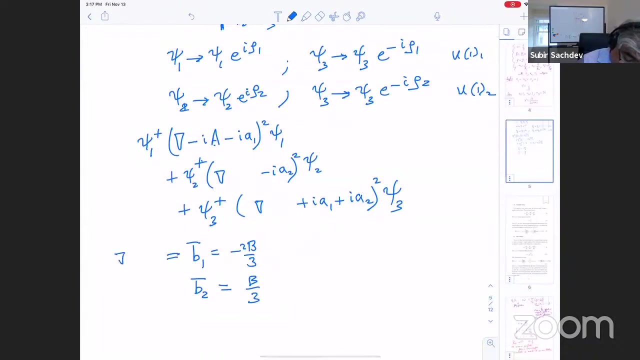 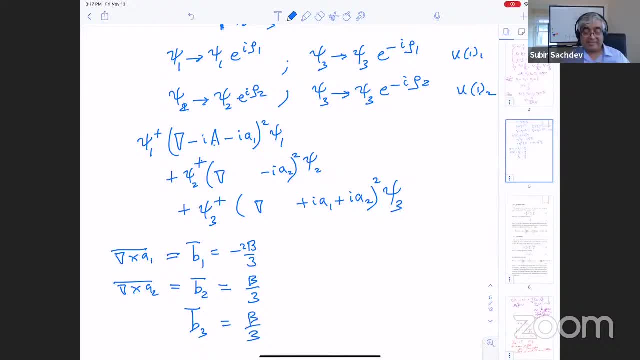 Okay, all is fine. Sorry. So this is the saddle point that we want to choose Saddle point. So we have these internal gauge fields, But now at the saddle point, unlike anything we've met before, These internal gauge fields have a non-zero value, non-zero magnetic field associated with them, so that in the end, at the mean field point, the total field that side one fields is B over three, which is A minus 2B, B minus 2B over three. 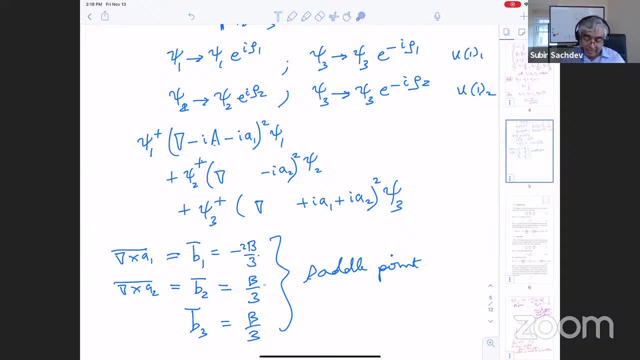 The total field that A2 fields is exactly B over three, and this is minus B1, minus B2, and that's also B over three. Okay, everything's fine, And then we have to do fluctuations about it. Okay, So that's our saddle point. 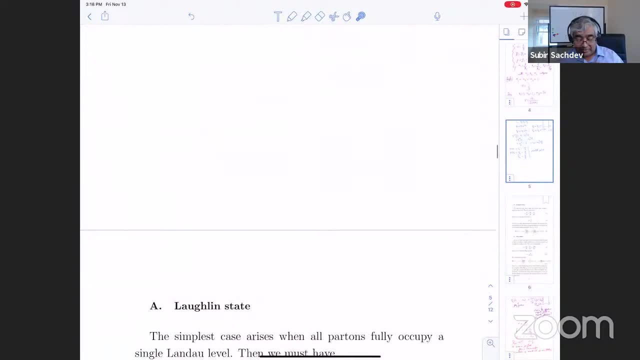 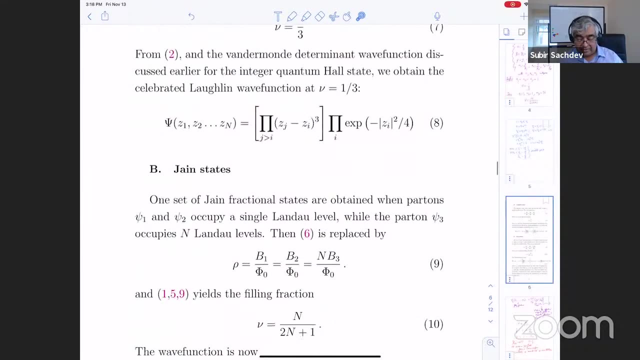 We're just, you know, turning the same crank. we have turned for spin systems all along, And so we have found a saddle point whose wave function looks like the Laughlin wave function. We'll talk about the chain states later. It's a little bit more complicated, but the same general idea. 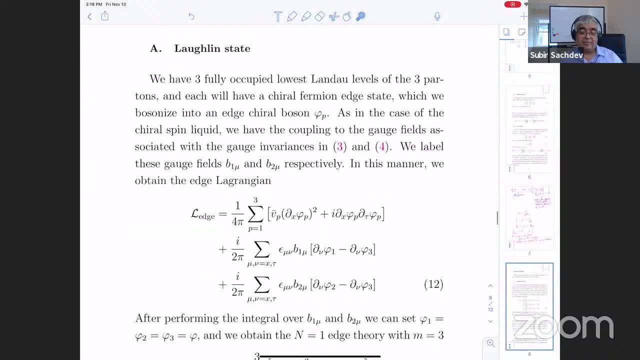 Okay. So now we want to look at the edge states, And I will look at the edge states. It's a little simpler than looking at what's going on in the bulk, which is a bit more complicated to straighten out. So how do we think about the edge states? 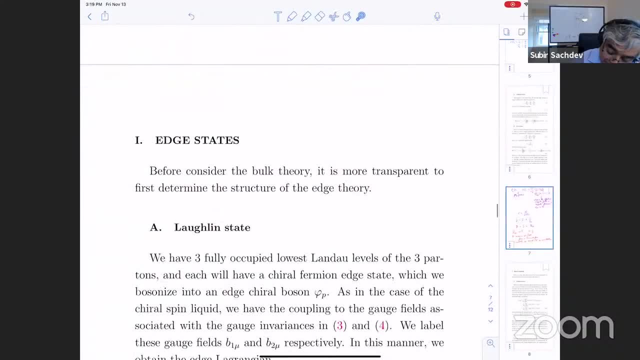 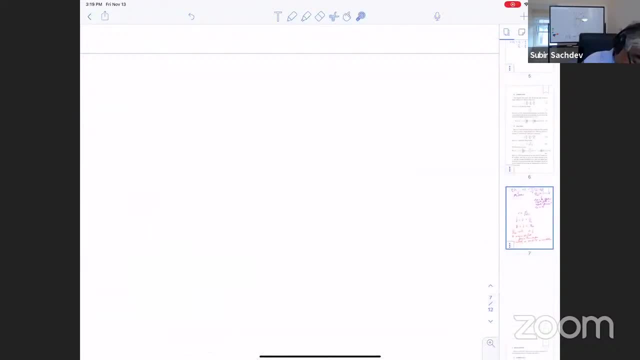 Well, for the edge states, what we're going to say is the following: Let's add a page, So we have the partons. So if you have parton one, so that's going to have its own edge states. So this is parton one. 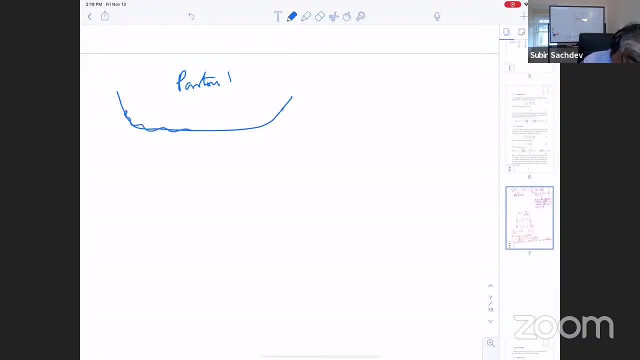 So this is described by some edge states over here, And these edge states are going to be chiral boson, because it's just a Landau level. So I'm going to have some chiral boson phi one And I have parton two. 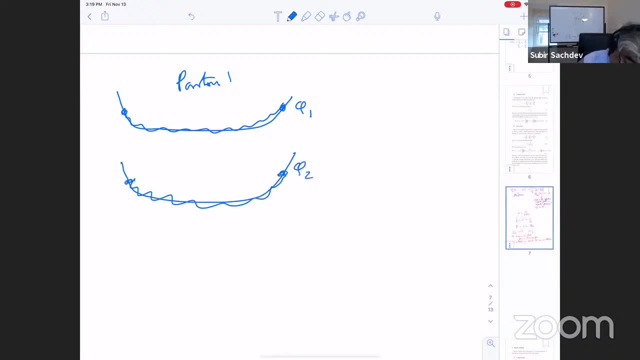 So that's going to have chiral boson phi two, And then parton three will also have edge states with the Landau level occupancy And these fluctuations here will be chiral boson phi three. So I'm going to have three chiral bosons on the boundary. 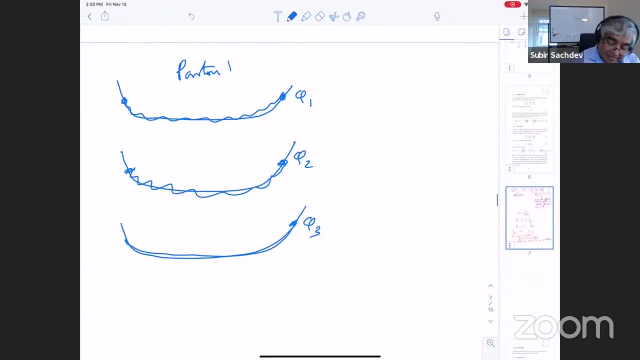 But then I also have some constraints. I have a constraint in the bulk, which should also hold, on the boundary that the density of the parton one must equal the density of the parton two, parton three, And this is associated with the gauge field. 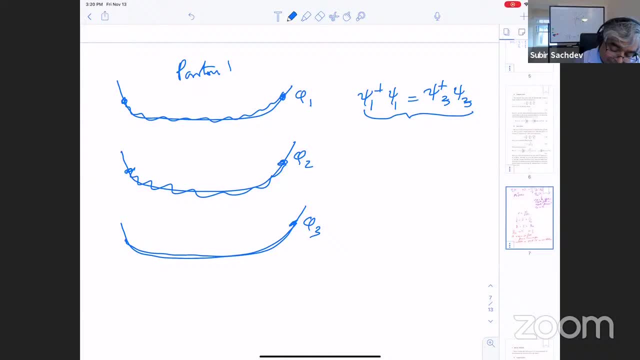 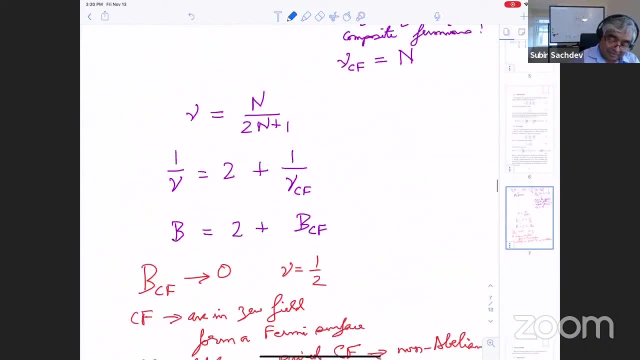 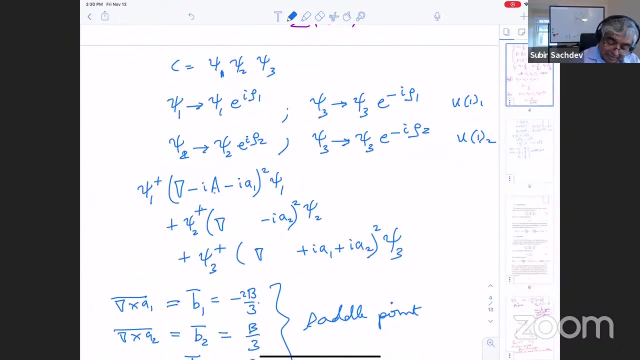 which is what I call. unfortunately, I call A1 on my written notes and B1 in the printed notes continue the written note convention. So here, yeah, this A1 acts with the opposite sign on psi one and psi three. So it basically imposes, if there's no Maxwell term for A1,. 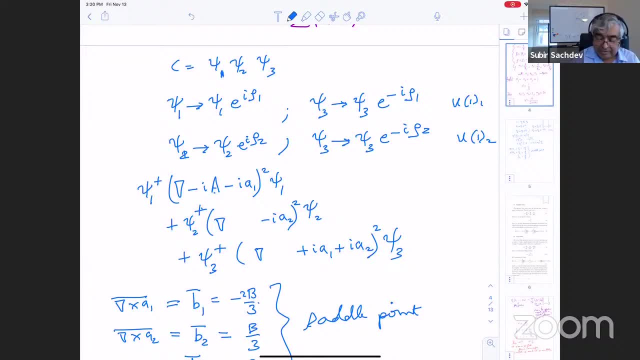 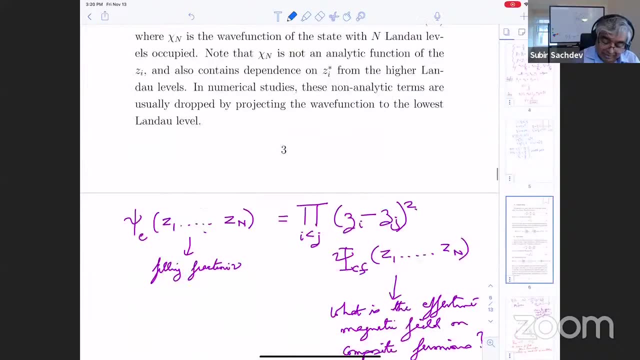 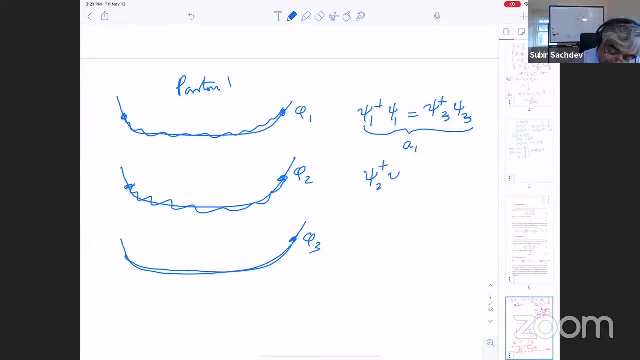 the equation of motion with respect to A1 imposes the condition that the current of psi one, A1, equals the current of psi three, And the zeroth component of the current is just the density. And then there's another gauge field: psi dagger two, psi two. 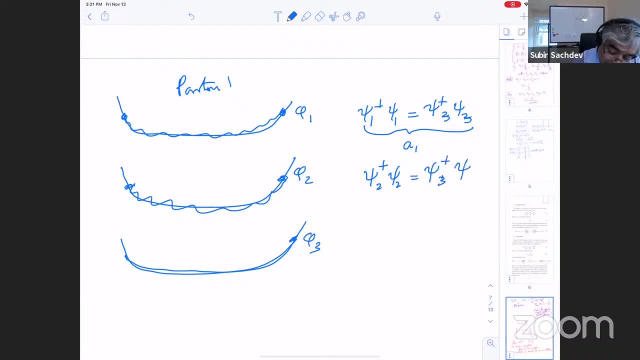 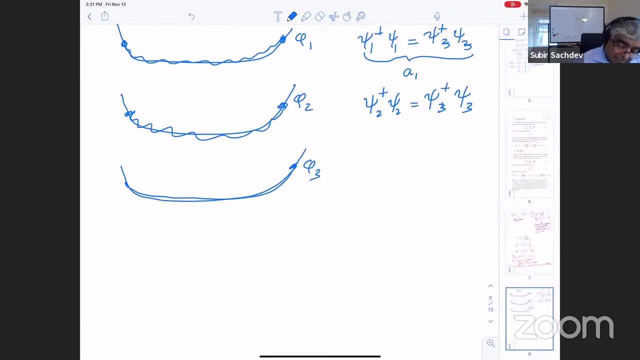 which imposes a condition that these two densities are equal. So now I can write down the boundary action. You've got the usual one over four pi of the three chiral bosons, So there'll be, let me just only write the kinematic term del x phi one. 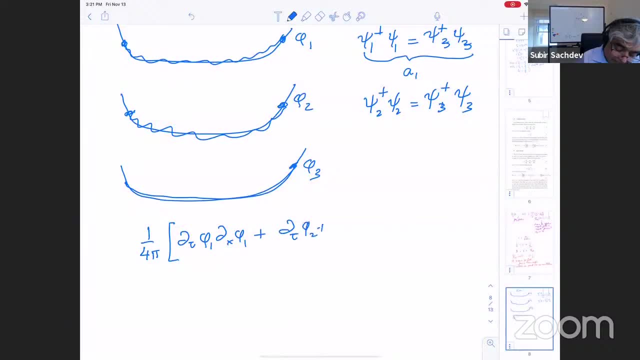 That's del tau pi two times del x phi two. That's delta phi three del x phi three. And then I have a constraint, And let me only worry about the density constraint. So the density constraint is: I A tau X must say the density of psi one must be equal to the density of psi two. 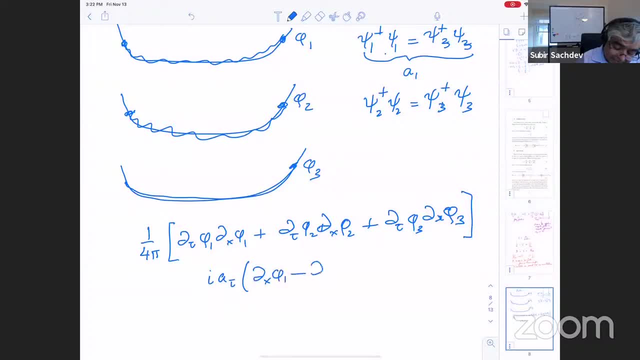 But the density here is just the derivative of phi one divided by two pi. So this oops over two pi. So when I integrate over A tau I get a delta function which imposes the equality of the density of psi one and psi three. 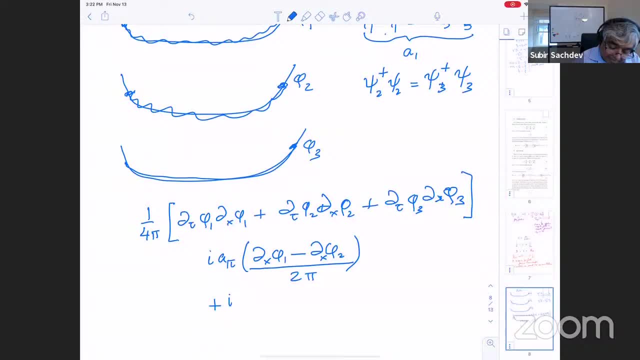 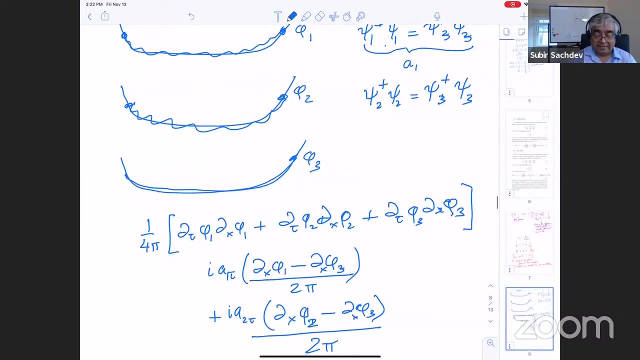 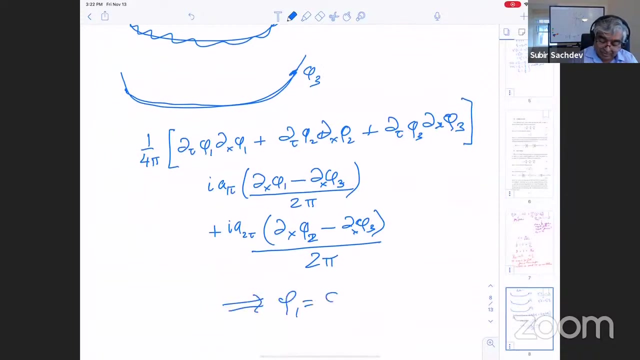 And similarly I get another delta function That's A1 tau, This is A2 tau of the density between phi two, And that should be three here. Okay, So that pretty much tells me that now I can solve this constraint. It just tells me in the end that phi one equals phi two equals phi three. 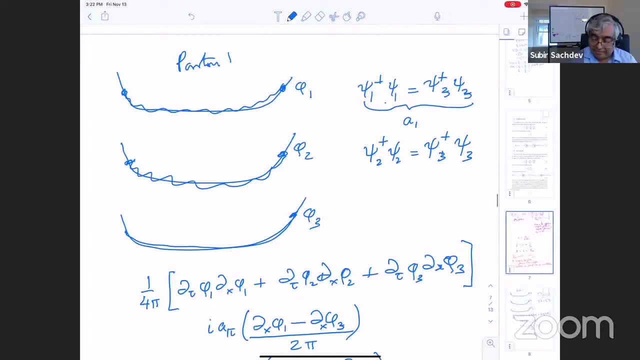 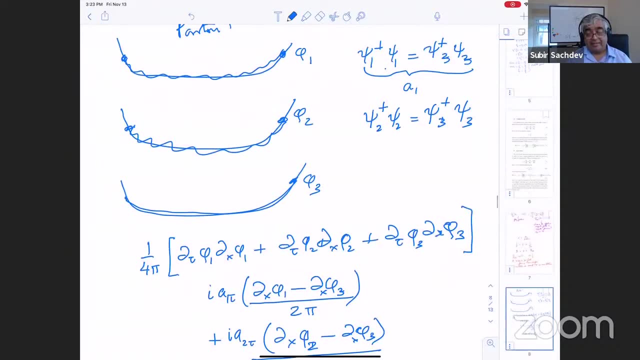 So it seemed as I was getting three different chiral edge modes. In fact I don't. I only have one of them. I have only one of them, but its coefficient is larger by a factor of three. So that's the final story. 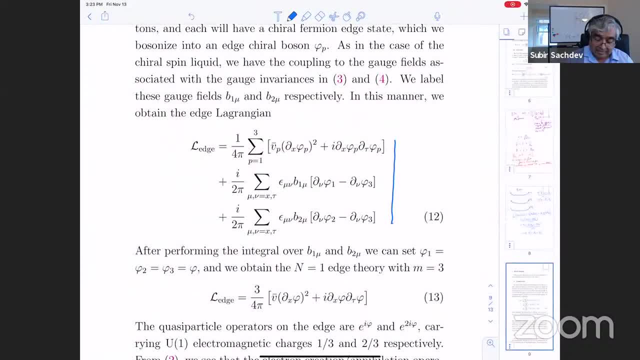 So here is the same thing written out more explicitly, And then you just put phi. one equals phi, two equals phi, three equals phi, And there's your answer. So the edge theory is: It is M equals three, It's level three as it's sometimes called. 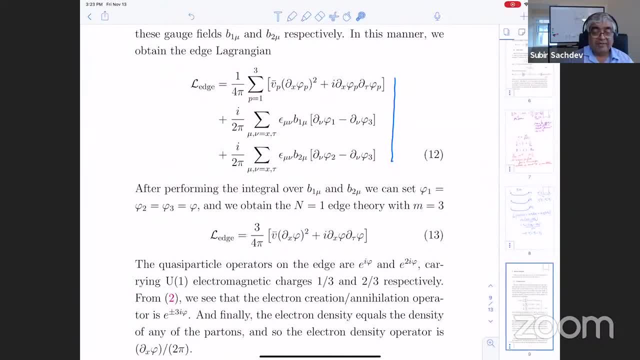 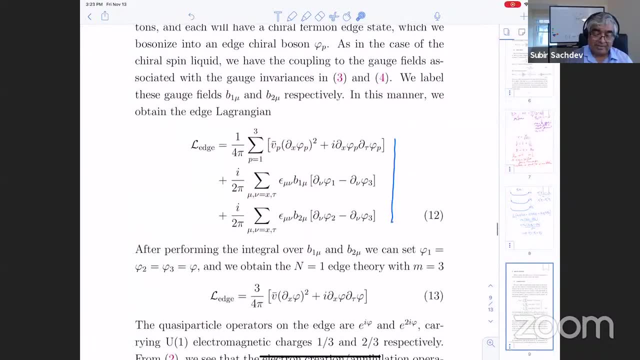 And this describes the excitations on the boundary, The quasi particle. what is the main excitation? Well, the excitation of the bulk are the partons. I can take a parton from one Landau level and put it to some higher Landau level. 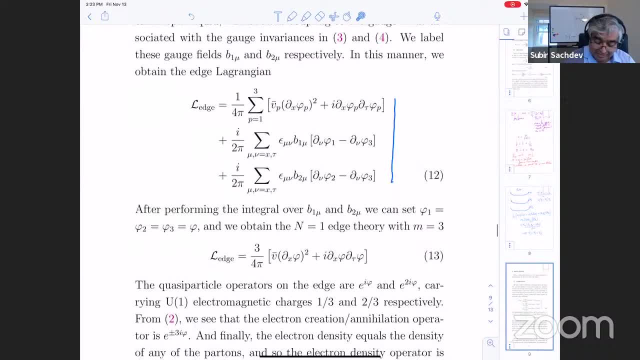 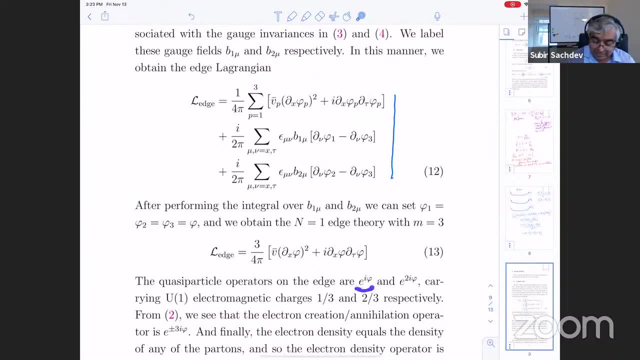 And the parton operator on the boundary is basically e to the i phi one, or phi two or phi three, But they're all equal And so it's e to the i phi. So that's my quasi particle operator, the elementary quasi particle operator. 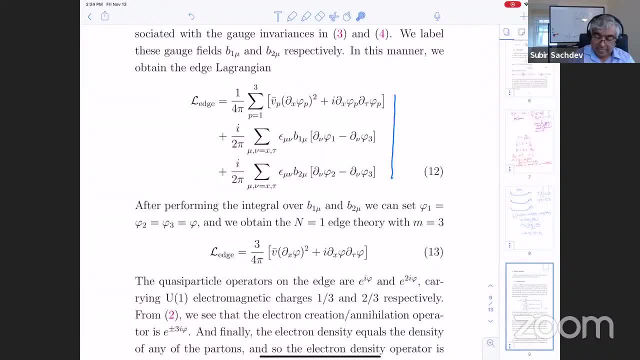 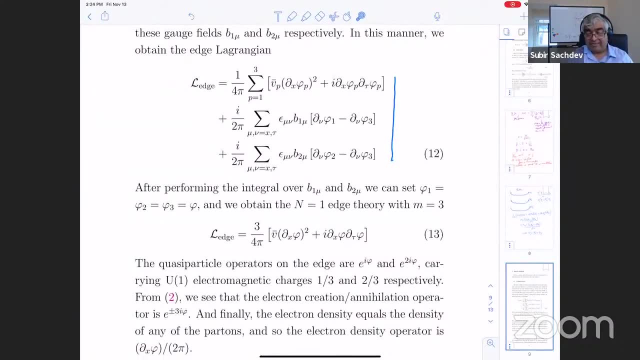 I can, of course, take two of it, And then, if you take three of them, well then you just get the original electron, because the original electron was the sum of three part, was the product of three partons. OK, so, once you know this and you know these are the, this is the bulk theory, these are the, the parton. 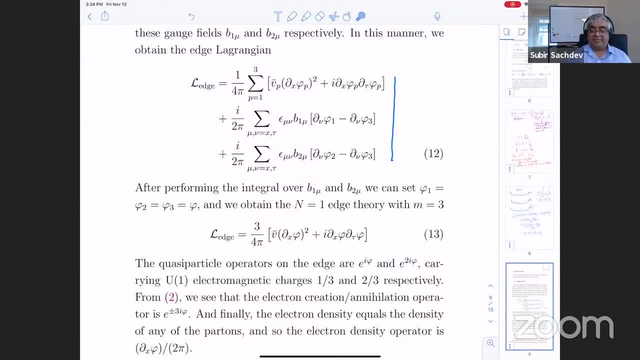 The quasi particle operators on the boundary, you're pretty much all set. Everything has been worked out in the chapter in Simon's theory, And so what you learn is that these, this quasi particle carries, charge one third, And it has anionic statistics with the angle pi over three, and so on and so forth. 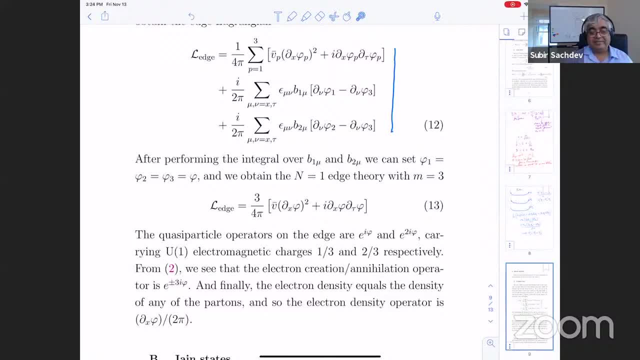 So it can work out all that. We've already worked out all the correlation functions And if you were to talk yesterday The experiments in your Kirby Kim labs, you know they were using theories of this type to describe the edge states of the fractional and also integer corner of all states. 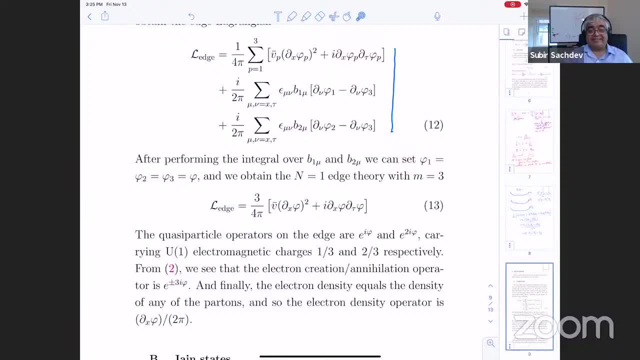 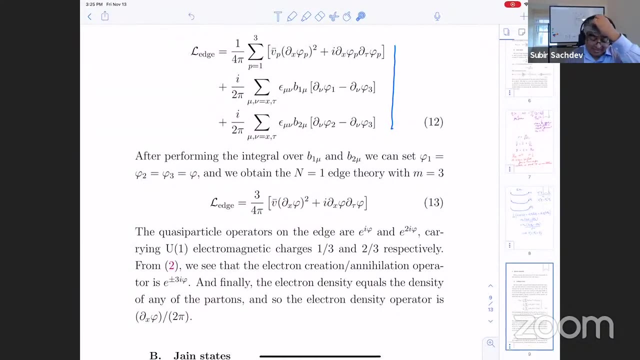 Yeah, so that seems you know I'm suddenly within two sentences. I'm just coming to conclusions that took the community many years to get. But I can do it because you spend the time playing all the groundwork, Learning about fractionalization and learning about John Simon's gauge theories. 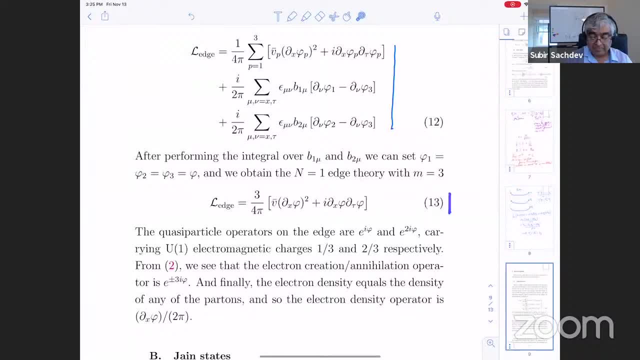 And once you put it all together it's really extremely simple: Any questions. And so it's probably. It's very like a freedom of choice or something, I guess. But I'm kind of confused by that. And why do you let external field be discounted? 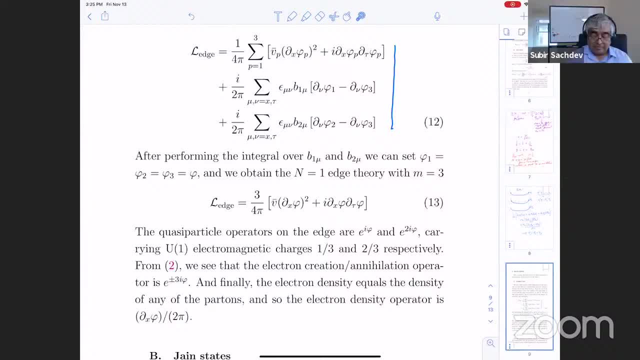 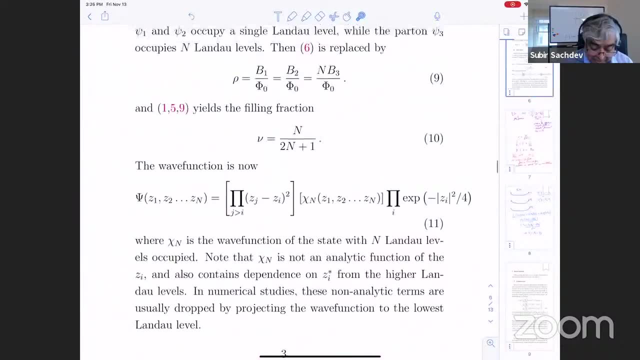 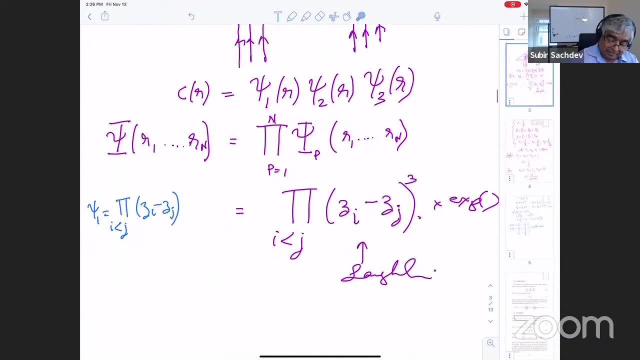 Only to one of them. Well, I mean, Maybe you can think in terms of gage transformations. So the couple of the external field is described by the gage transformation. So there is a global gage transformation where see? so let's see. 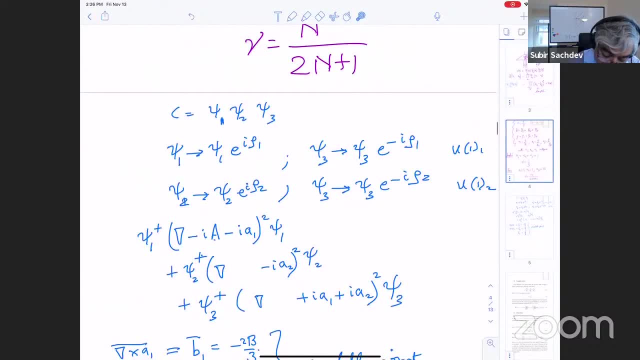 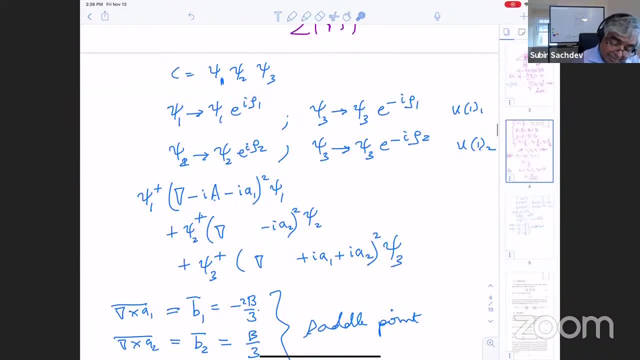 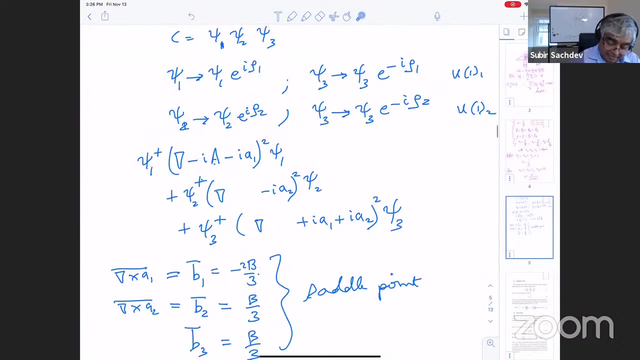 I mean you can couple it Any way you want. I'm kind of reluctant to let me write it over here. so these gauge transformations I was writing down were the internal gauge transformations. so these transformations are the internal ones. there's one more gauge transformation. 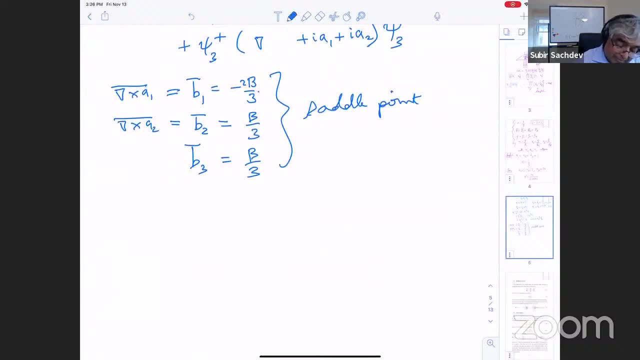 which is the external one, having to do with the physical electromagnetic gauge invariance, and that is C, goes to C times E to the I chi. so this tells me that under this external, this is U1 X. so under this external gauge transformation, this tells me psi 1, psi 2, psi 3. 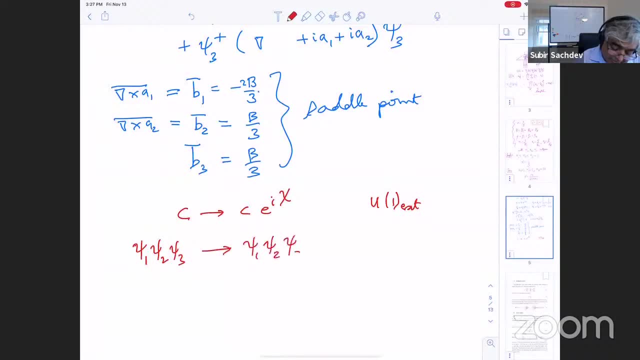 goes to psi 1, psi 2, psi 3 E to the I chi. so it's up to me. I can take this chi and split it into three ways any way I want, but that's usually bad practice because sometimes you have to worry about. 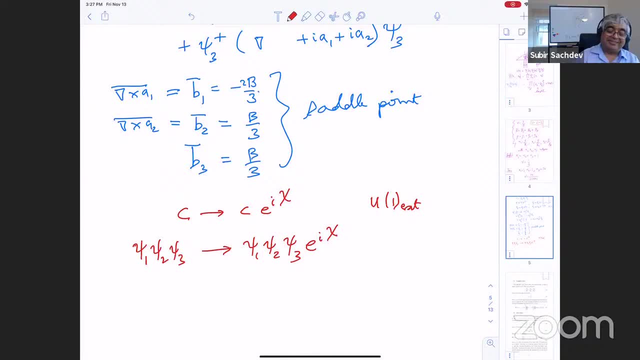 you want to keep all the charges integer. you don't want to, because that affects the quantization of various scalar fields you're going to get. so it's always good practice to keep things integer, so what I chose was to put this chi transformation entirely onto psi 1. 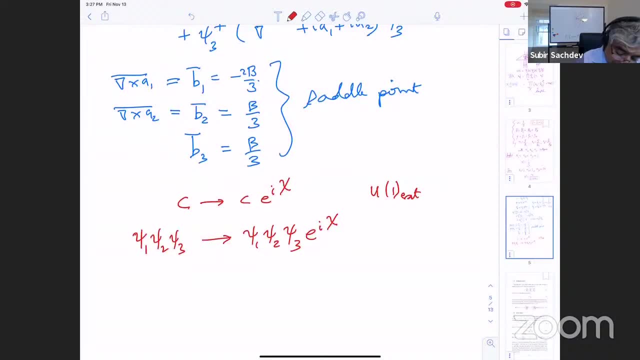 so now, under all the gauge transformations, I conclude that psi 1 goes to psi 1 times E to the I chi, plus E to the I rho 1, psi 2 goes to psi 2 times E to the I rho 2 and psi 3 goes to psi 3. 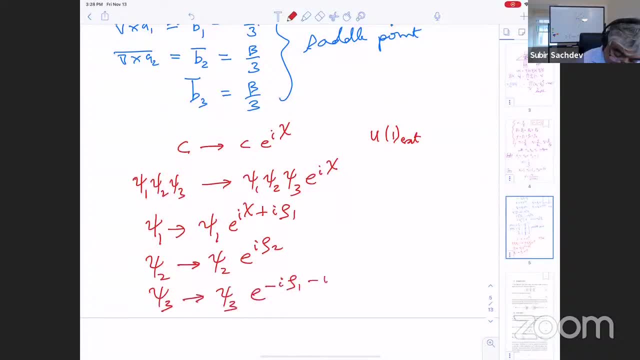 times E to the minus I rho 1, minus I rho 2. so this is our actual full gauge transformation, including the external one, so I've just chosen to put it over there. so this is how I define it. and then, once you have this gauge transformation, 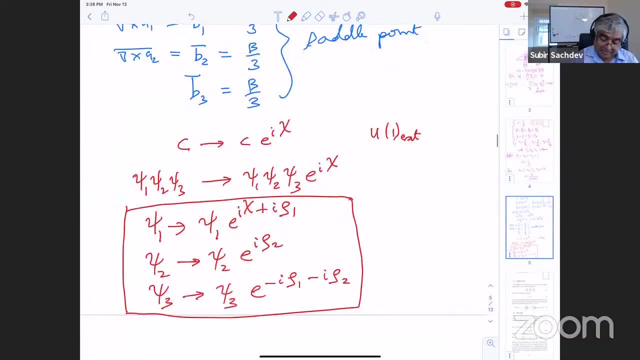 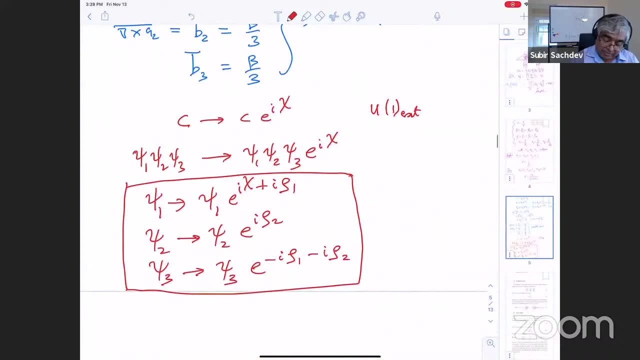 then the coupling to the external field is pretty much fixed. so basically you have to put the capital A over here to make the whole thing gauge invariant. but you could equally I'll have put chi over 3 for psi 1, psi 2, psi 3. 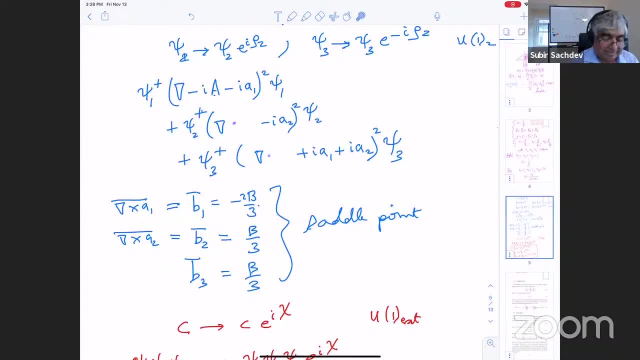 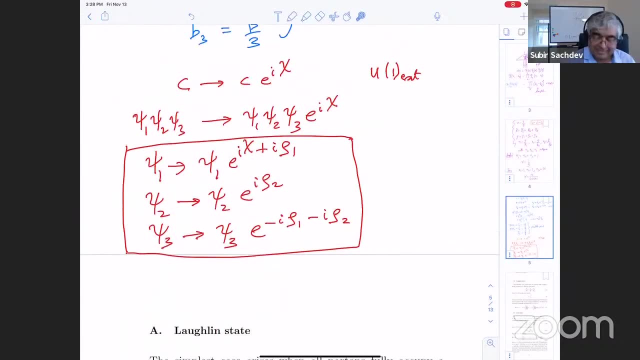 and put a field A over 3 in the different places. you could have done that. it's just a bit messy. I prefer to keep it like that. I prefer to keep it like that. I prefer to keep it like that. I prefer to keep everything. integer, that's all. 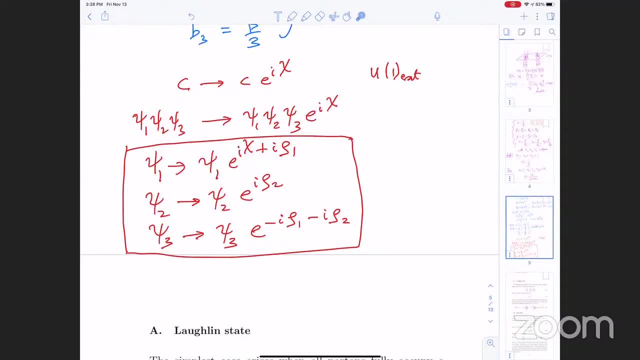 I see, I see, thank you. I mean, the main point about this, this transformation that you see from here, is that the total field, that each that acts on all three particles is always just capital B. that's the important point, because the rho 1 field always cancels out. 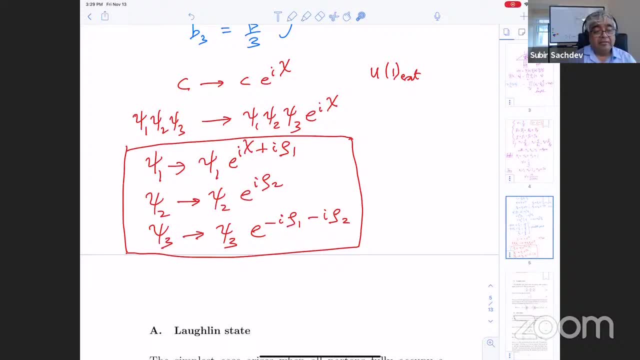 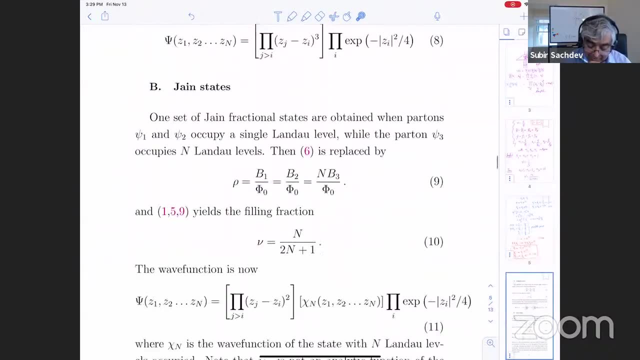 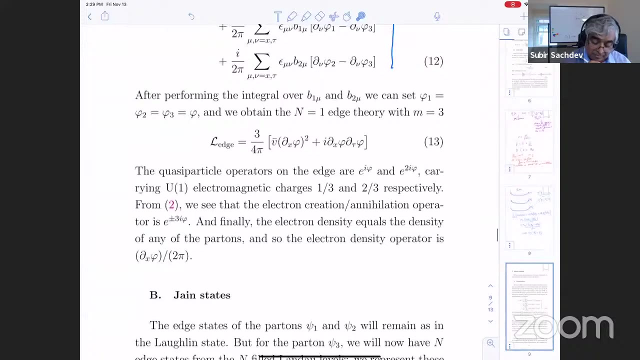 the rho 2 field also cancels out, the rho 1 field also cancels out. so thegue I use here is: is the base to the the of the state, of the state of the state, okay. so I say, let's do the same here, let's do the same here. 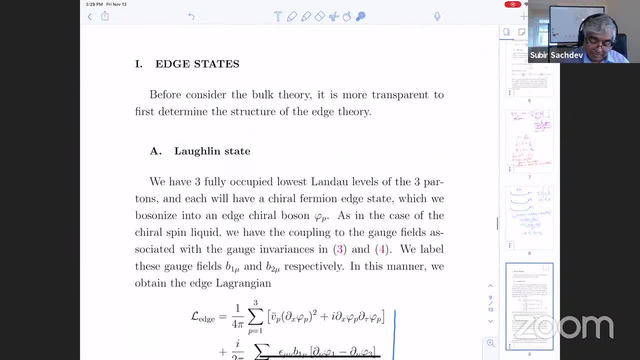 OK, so let's play the same game now on the boundary. sorry, in the bulk for the Laughlin states we've done the edge states, so I guess in the notes we do it the other order. so I guess in the notes we do it the other order. 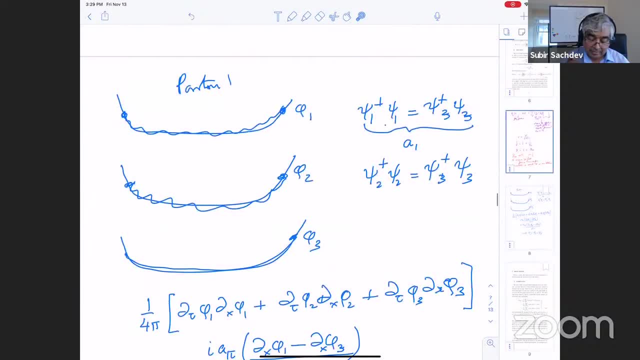 so let's do it for the Jane states. so let's do it for the Jane states. what's going to happen? well, in the jane states, you're going to get n partons of parton three. so you're going. so you're going to have more partons here. 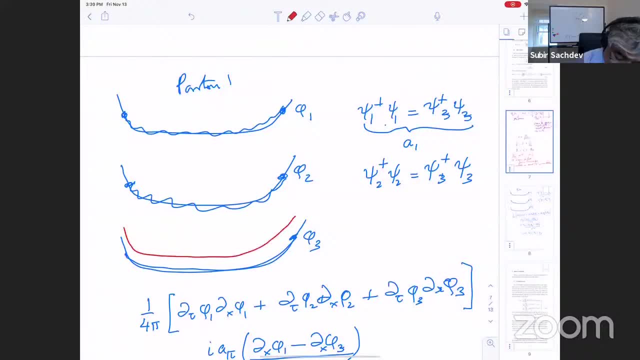 because you're occupying many landau levels of parton three. okay, so how do we? so? for each one of these landau levels there's an edge state. so what we should do- and we only need to, you know, we only know how to work with free fermion edge. 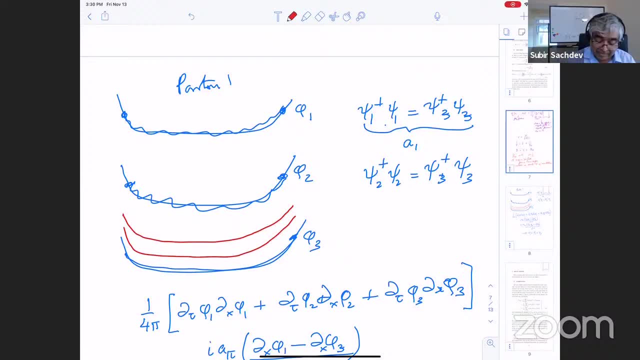 states to begin with. so basically we have a free fermion edge state, chiral edge state, for every landau level. uh, you know, one here, one here, one here. so basically we are now we're going to get. in this case there are three, uh landau levels occupied of the parton three, and so we're going. 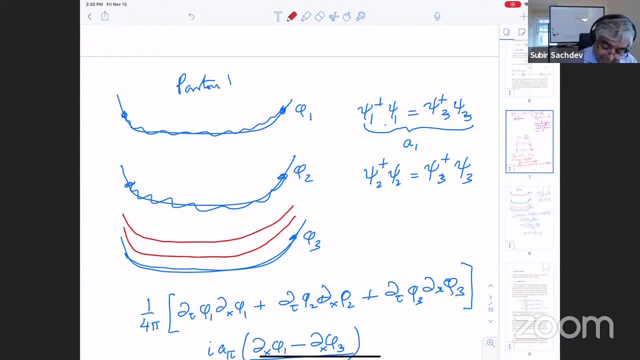 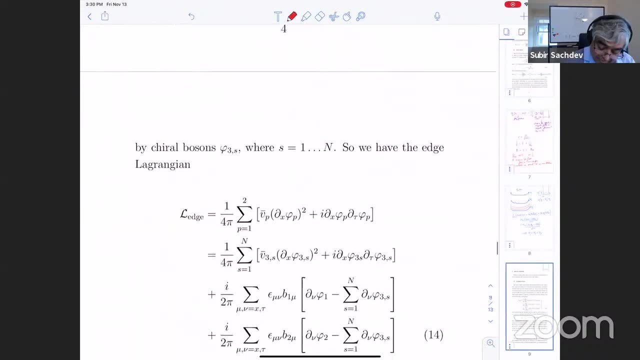 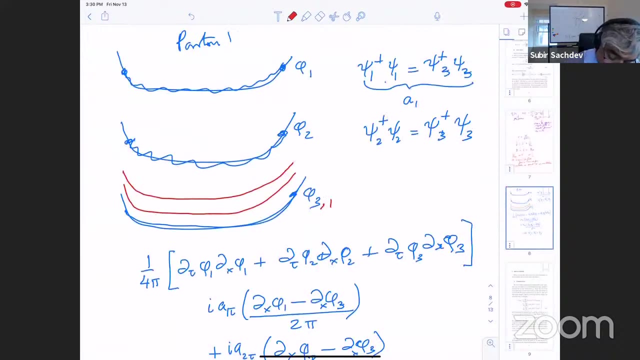 to get three, uh, three partons on this edge, and how do i label them? what label did i do used? yeah, so i call them three comma s, so there'll be three comma one, so phi of three comma one, and then i'll have phi of three comma two and phi of three comma three. 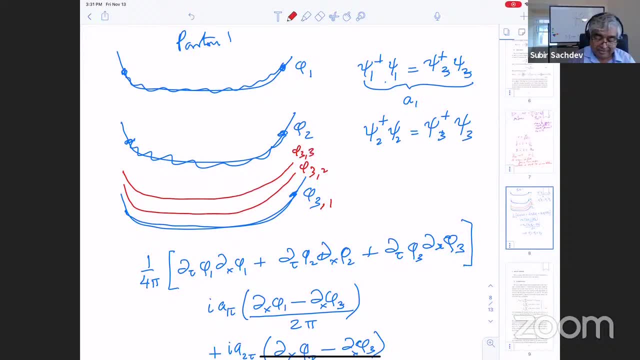 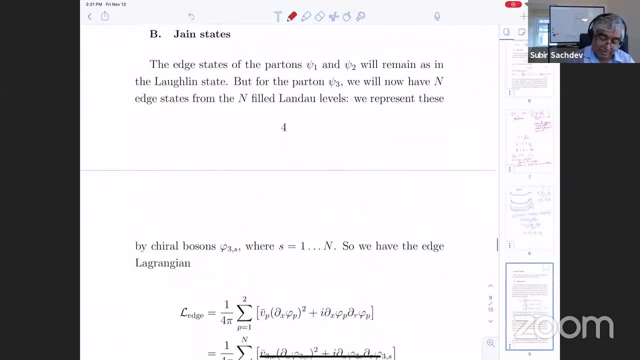 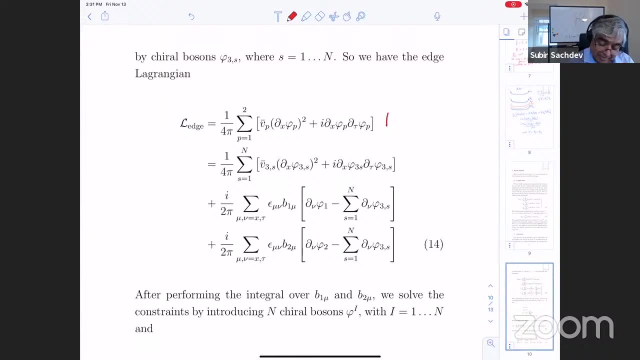 so i'll have n plus two where n is any integer, uh chiral bosons in these higher states where one of the partons has a weaker magnetic field acting on it. so this is the first two, as before, and the third one has a sum over s going from one through n. okay, and now i have to put the density constraint. 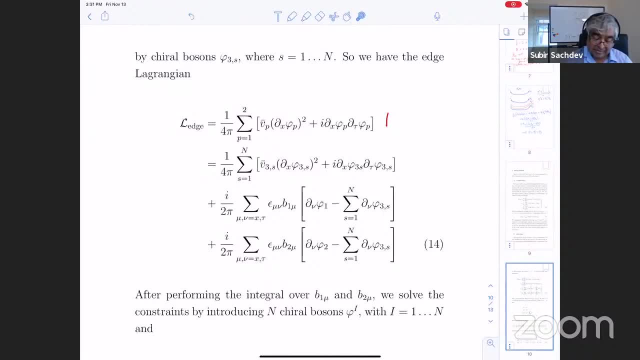 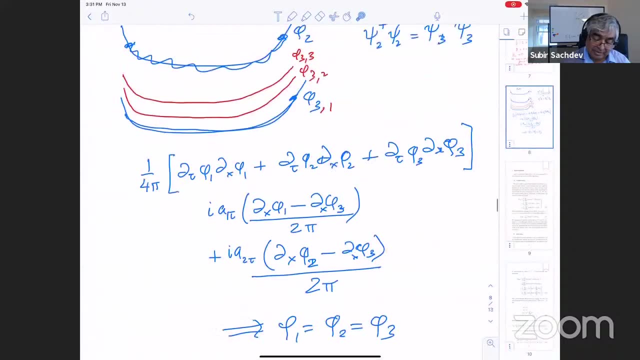 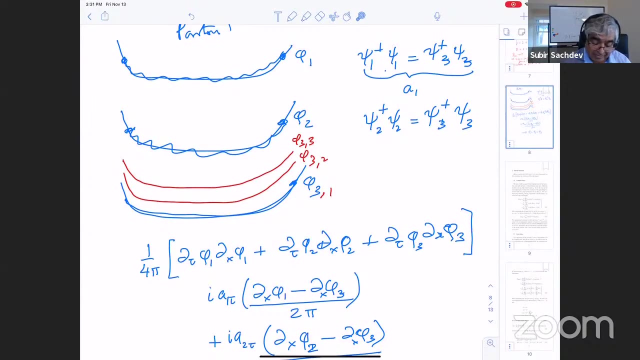 and now there's a difference. uh, the density constraint is really on the density, uh, the total density. so the constraint is that the total density of fermion three must equal the total density of fermion two, because it's it's the same partons that are going back and forth. 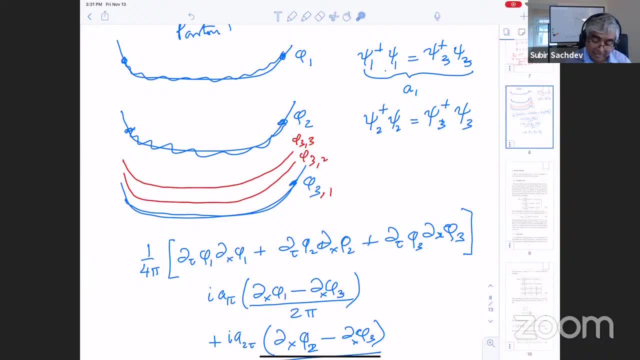 allowed to go back and forth between all of these edge states. so, even though they're described by separate chiral bosons at the edge in the bar, that their constraint is on the total density. so, therefore, when i put the constraints in terms of these conjugate gauge fields, so these are the 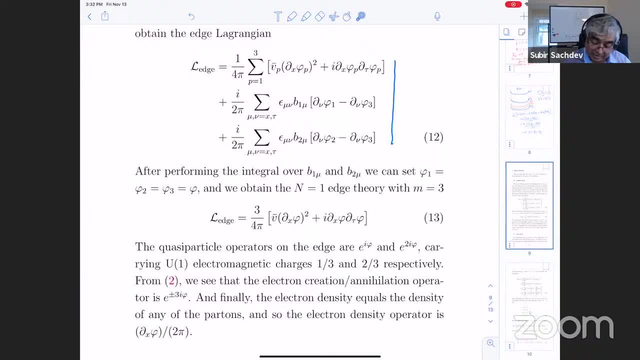 constraints here for the laughlin states. uh, it's exactly. there's again only two gauge fields. so the number of partons- the number of partons is the number of partons that are going to be- the number of sorry chiral bosons- has increased, but the number of gauge fields has not, because 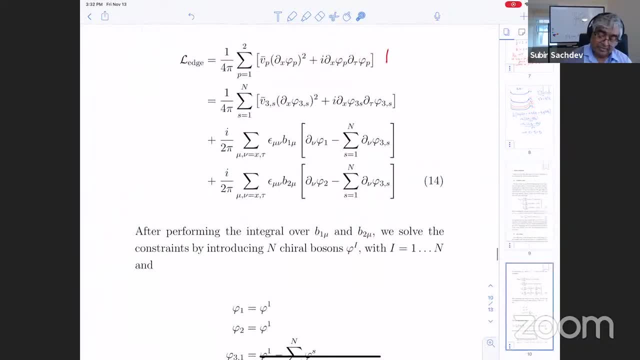 the number of constraints was still the same. uh, so therefore i i basically have to put in the sum over the phi's here with these two gauge fields. okay, so now i have a new situation. i have more. you know, i have n plus two chiral bosons. 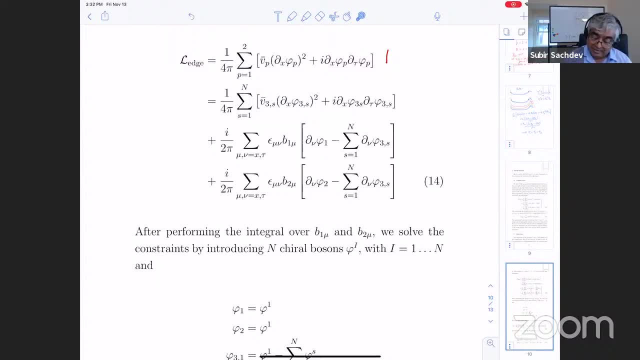 and two constraints. so that means i'll be end up with n chiral bosons. so there, now you see an example of how you get more than one uh, chin simon's gauge field or chin simon's uh edge state here. so now you could have more than one edge state. uh, even, yeah, yeah, even in the, even in the. 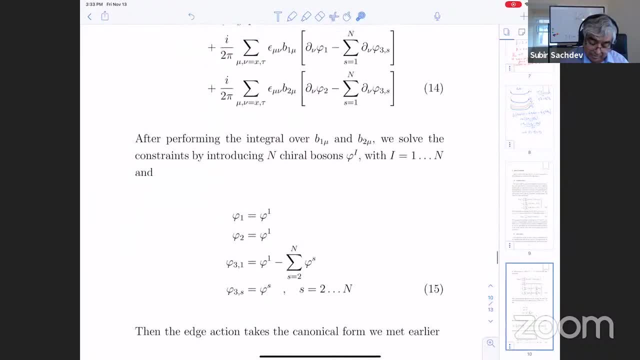 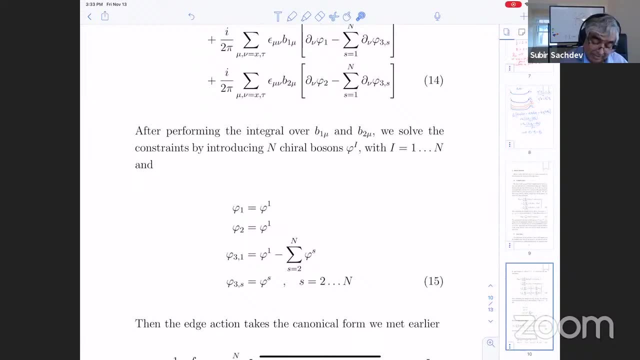 lowest land or level for this chain state. so so, basically, i have to solve, i have to write the n plus two constraints and n plus two chiral bosons in terms of n fields, uh. so there's some choice on how you, how you pick those, um. so what i've done here, uh, is that i take: phi 1 equals to phi 2. 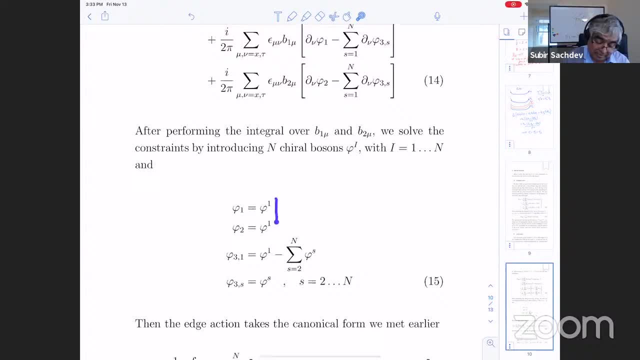 because that is one of the constraints. so that's just one field here. and then phi 3, phi 3 s from s going from 2 to n. i just say it's phi s and then phi 3- 1. i take as this difference, so that the both constraints are. 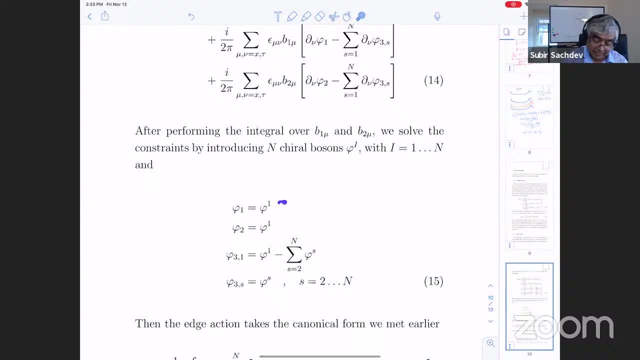 satisfied, so. so this is equal to this, and the first one is equal to the sum of all phi 3's. um, yeah, okay, and this is just one way of doing it. again, i like to solve the constraints so that i i only have integer coefficients. if you start having fractional coefficients, then 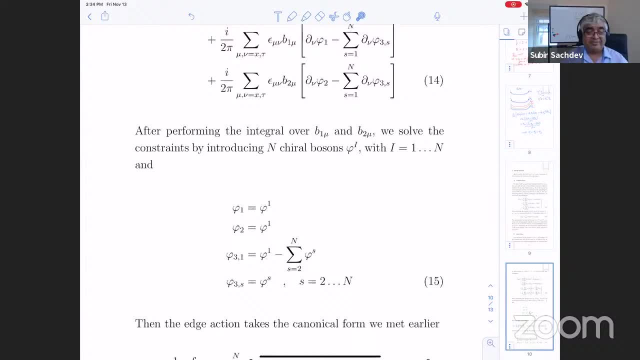 you know, like more complicated later on. we don't want fractions here, so you just want integers, and so now you substitute this back in here with this change of variables. there are other choices you can make. so that tells you that in fact, the k matrix that you're going to get is not unique. 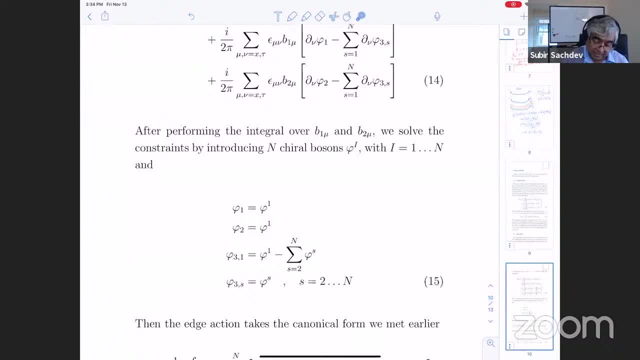 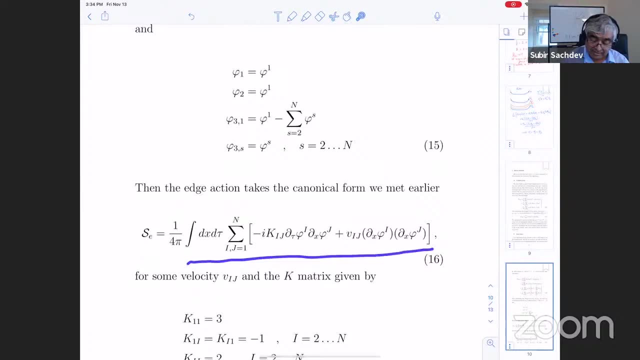 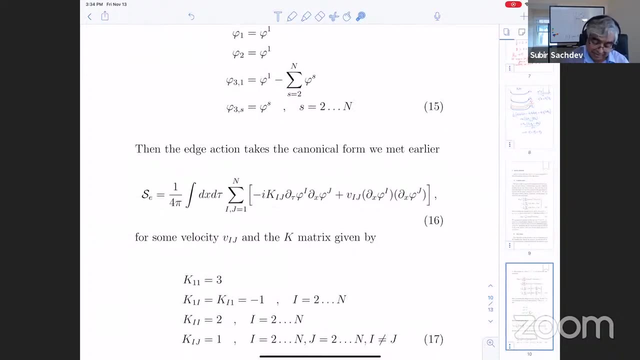 you can always take linear combinations with integers and get other k matrices, and when the death circles? now you get our very general edge theory with n, uh, chiral bosons. and what is this k matrix? well, you can just work it out and here are some pictures of it. this is: 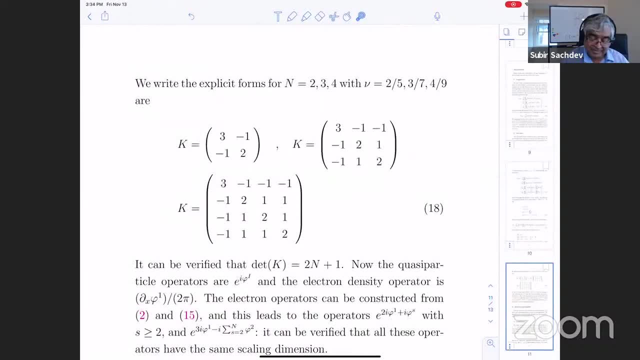 what it looks like. it's um, uh matrix, with integers in it, uh, corresponding to our solving these constraints. so now, this is, you know, quite a non-trivial thing. we wouldn't have been so easy to guess this. uh, and and from this now you can you have different types of quasi-particle operators. 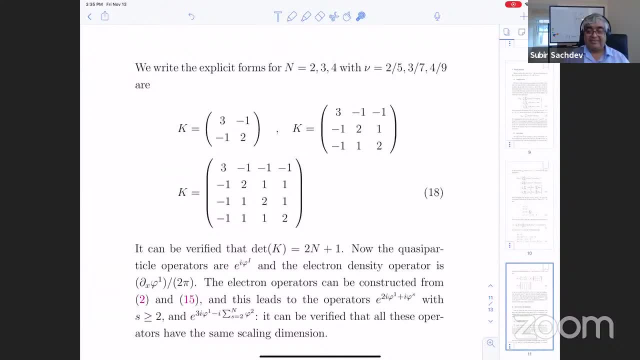 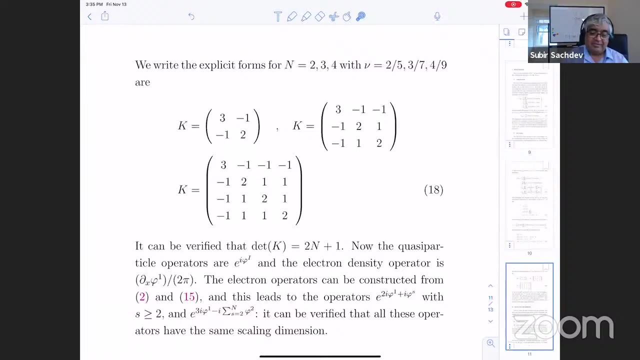 they have different densities and different statistics and you know it can become quite a messy thing, And yeah so. but now you have a edge theory. for example, the two fifth states when n is equal to two, or the three seventh states when n equals to three. 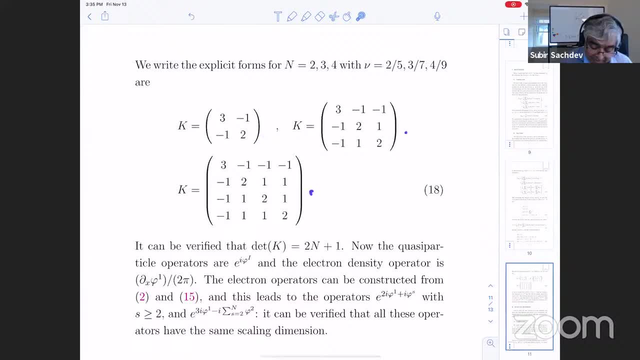 This is the two fifth states. nu equals two fifths, three, sevenths, four, ninths all of and these states are seen. I don't think the edge states of these hierarchy states, these higher states, have been measured that carefully. 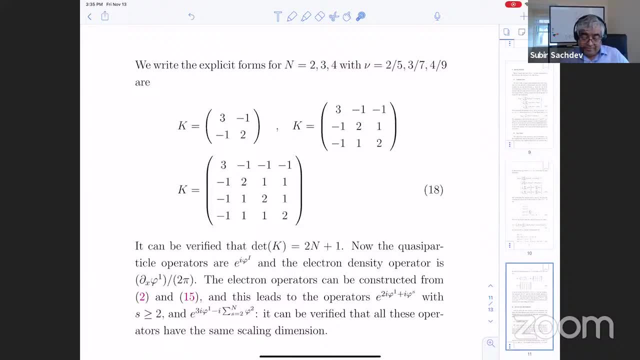 mostly at the nu equals one third level, But anyway. so those are the famous Jane states, And that pretty much completes our description of almost all the observed fraction quantum Hall states. The prominent exception that we haven't discussed is the gap states. So, for example, we have a state at nu equals one half. 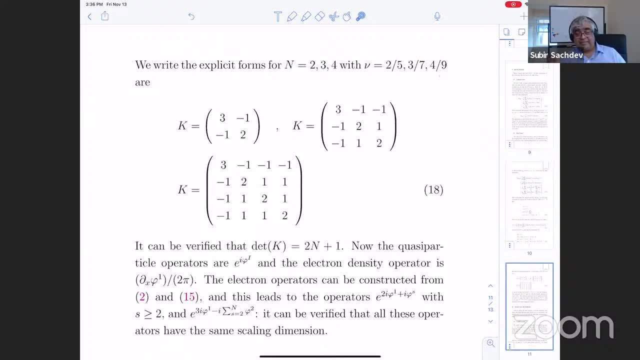 All of these states here that I've described have all denominators, but there are some states that even denominators and they correspond to pairing of the partons, And I'm going to describe an example like that in the next chapter, which is on the. 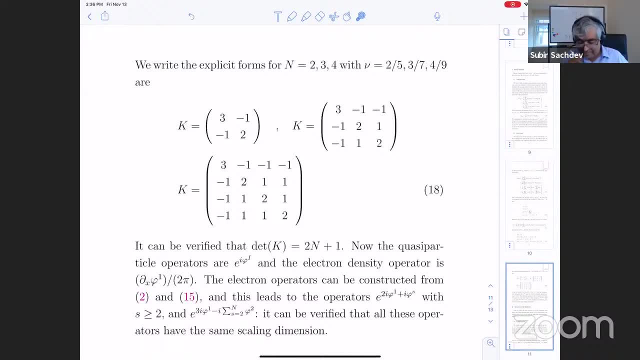 on the Ketayev-Honecker model, which is very similar to even denominator fraction quantum Hall states, But it's a bit simpler, so I'm going to stick to the to the Ketayev theory. All right, Sorry, can I ask a question? 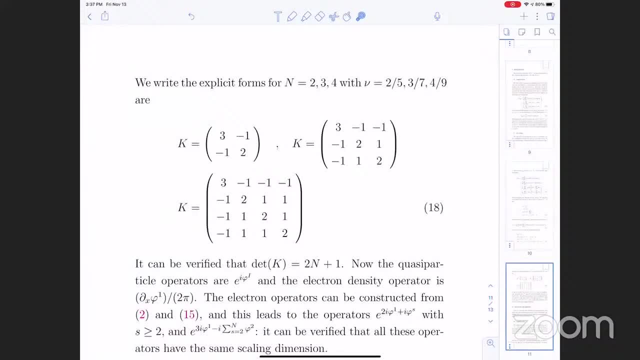 Yes, please. What is the interpretation of this determinant K here? I remember in Z to spin liquid was the torus degeneracy or something. This is exactly what it is here too. That's the determinant. So that's the degeneracy of the K. 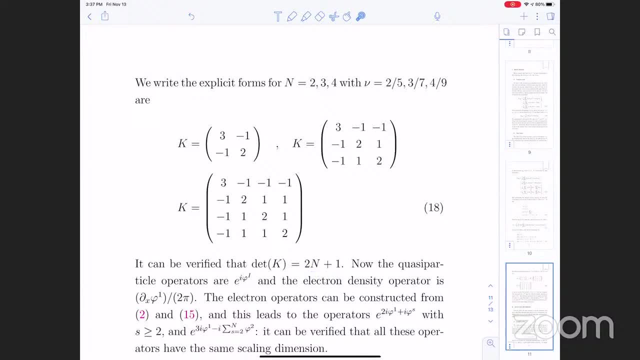 That's the degeneracy of these states. It's now a little bit of, quite a bit more subtle. It's not something you could have guessed, but that is the answer, That's the determinant that gives the degeneracy on the torus. 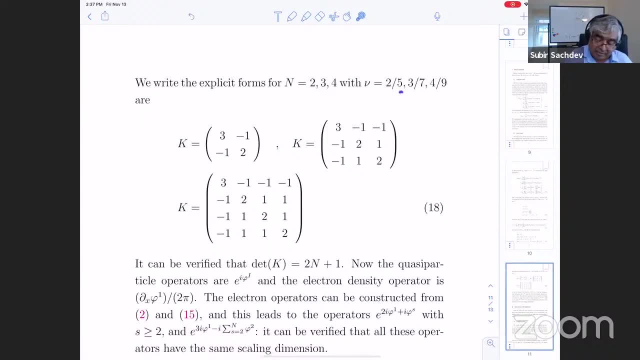 In this case it just turns out to be the first sequence of J and C, just the denominator here. So it's very similar to the Laughlin state also, which has degeneracy three And the degeneracy in other other spaces. 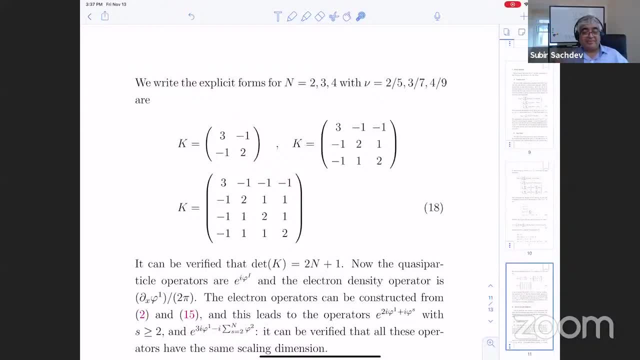 with higher genus surfaces is. I don't know. One can work it out from this K matrix, but I don't know what. the formula is off the top of my head. So so how do we kind of change how many Landau levels? 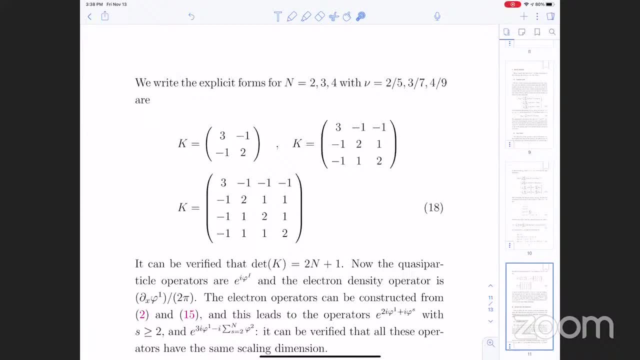 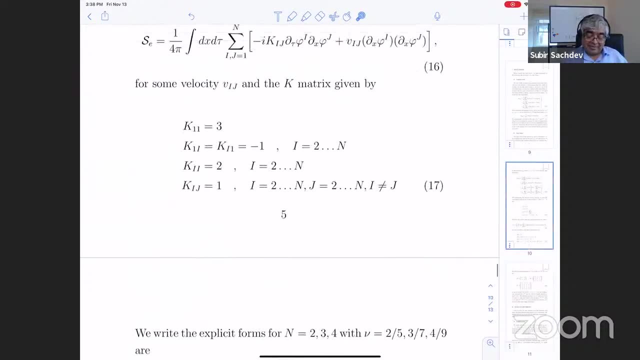 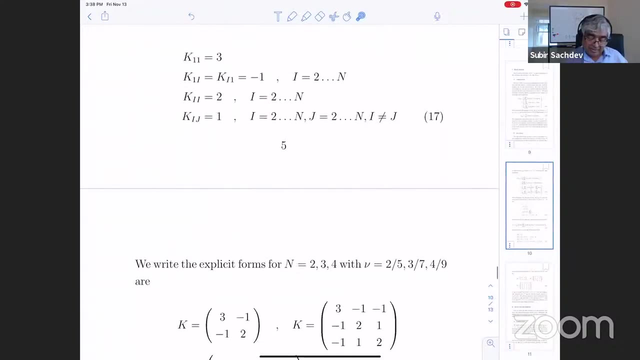 are filled for any specific parton Like: do we have any control over that in experiments? Control over it? No, not really. I mean the partons are theoretical construction, Right, That give us some. what we can observe are the edge states. 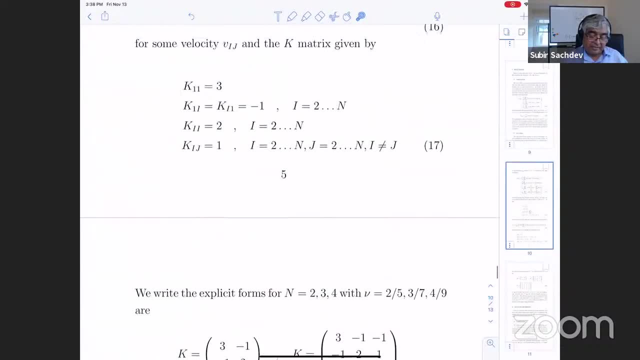 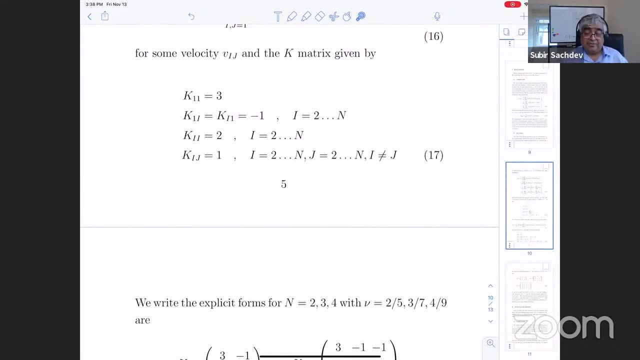 So so this is telling us that there are in this two fifth state, for example, there are two independent edge modes, because N equals two And that you can observe, You can look for this- two chiral edge modes with the properties. 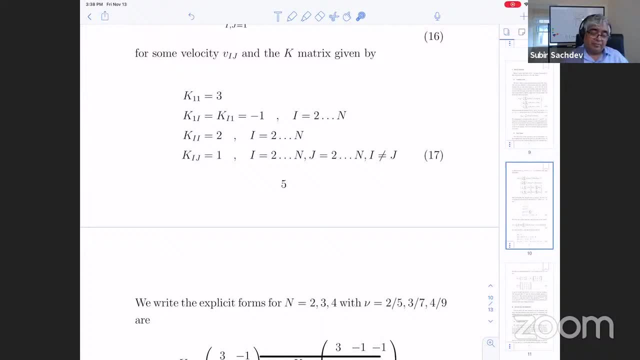 Described here. You also have to worry about the effects of disorder- And there is a lot of work on that which I'm just touching here, which does affect the edge modes and mixes them up in some interesting ways sometimes, But okay. 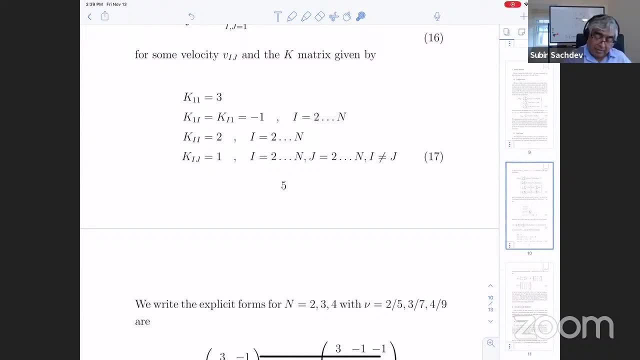 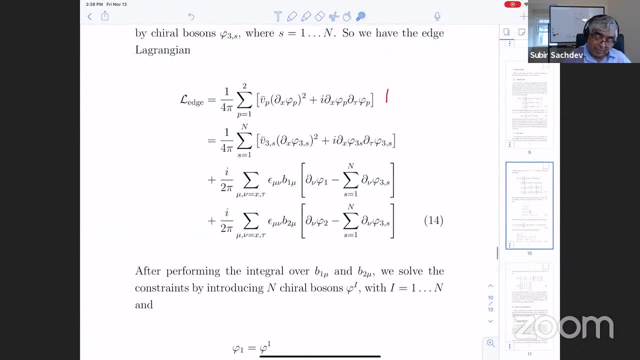 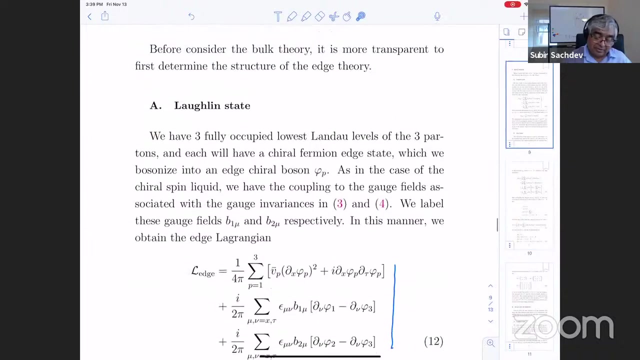 Ignoring that caveat. in principle this is observable. So the question really is: you know what is what determines what is the parton construction for a given filling fraction? There could be other partons construction you could think of And the answer is really: one doesn't know. 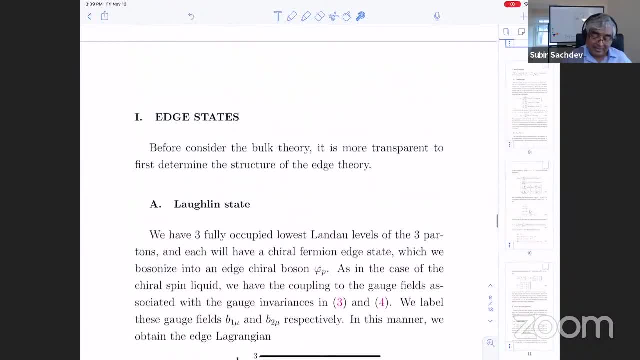 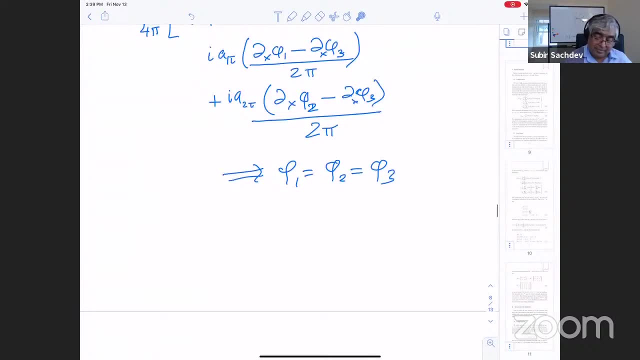 One simply has to look at experiments and see what fits, or one has to do some very complicated computer calculation to figure out which is the right parton construction. I guess maybe the better way to say it is that which is the right topological order. 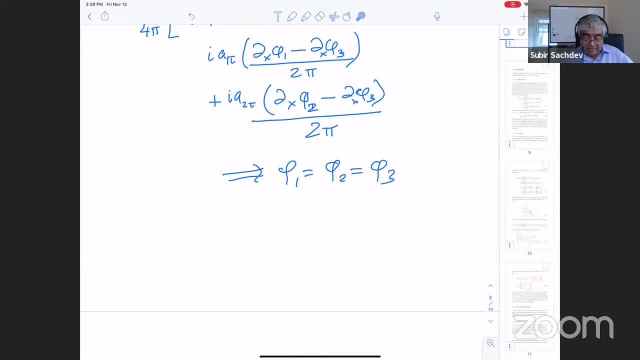 Which, in other words, what are the anionic quantum numbers? What are the anionic self and mutual statistics? What is the set of edge states, which are all, of course, closely related? So there's some invariant information and there could be more than one parton way of getting it. 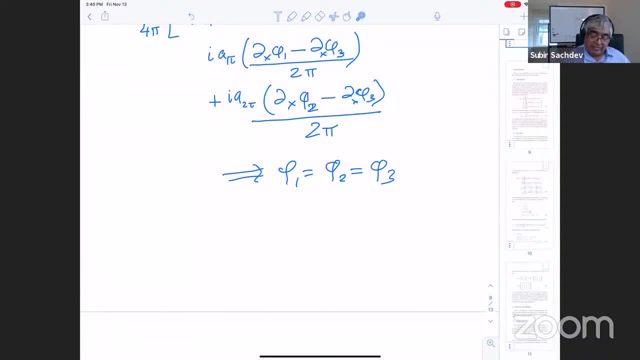 Well, that's yeah, But the two ways of getting it are just, you know, probably not an equivalent. There's just some gate choice that you're making, I see, And so, basically, if I take like some specific Hamiltonian or like a specific system and I do calculations, 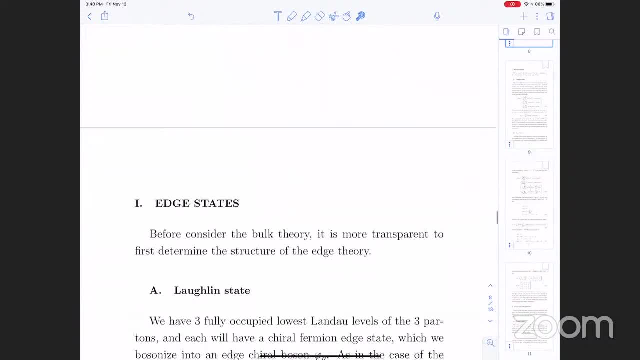 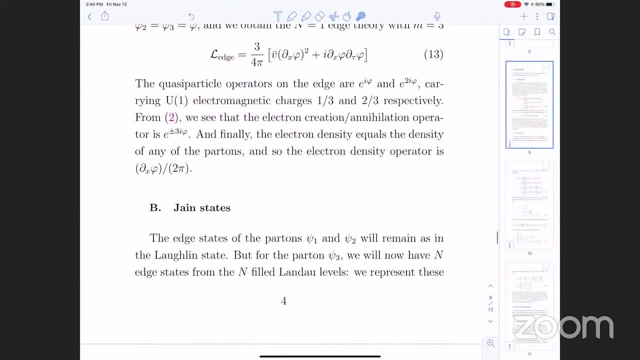 and I find like a lowest lying solution. and for this solution I kind of, when I do this, I find out like how many Landau levels for each parton. if it's like properly describing the system, how many Landau levels I'll field. 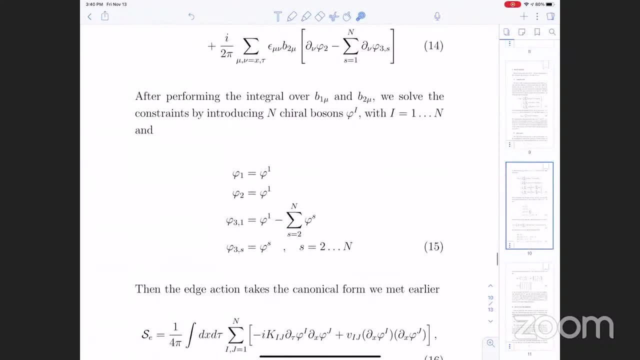 And then I kind of end up with like all these numbers like n being something. And Yeah, I mean the partons are kind of a gauge. They carry these emergent charges of emergent gauge fields, So they're not directly observable. 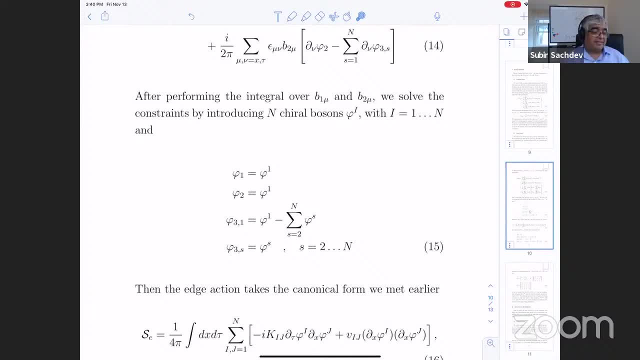 even in a numerical experiment. If you do some numerics you'll get out some energy levels maybe, and maybe that'll tell you about what's going on at the edge. And then you'll have to match the things you observe in numerics to the gauge. invariant observation quantities. 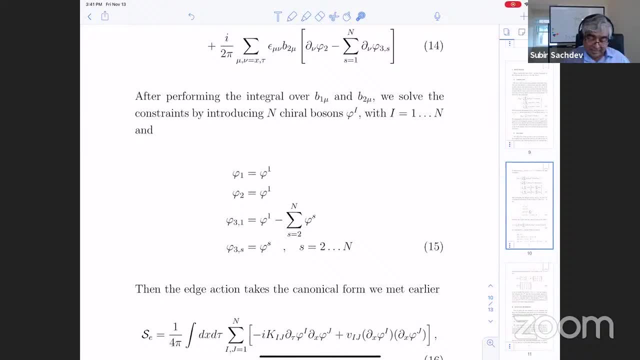 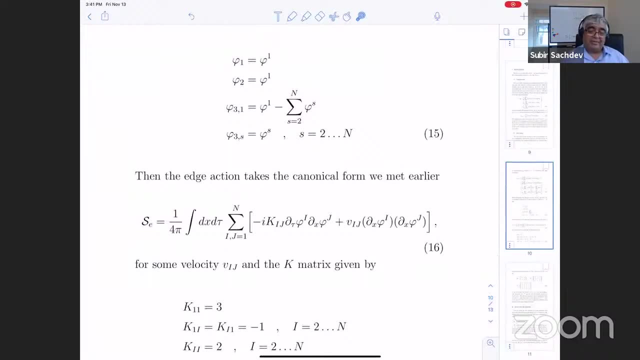 you have here from this calculation And the gauge, invariant quantities are basically the K-means, the matrix and the statistics and so on, and the degeneracy on various manifold and the number of quasi particles, their quantum number, I mean their statistics factors and so on. 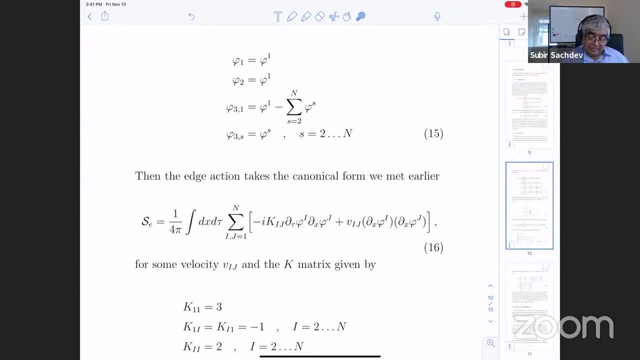 So that's the invariant information. The fact that I, you know, I had initially had n plus two partons and I ended up with n edge states that n plus two is not an observable quantity, It's just some gauge dependent choice I made. 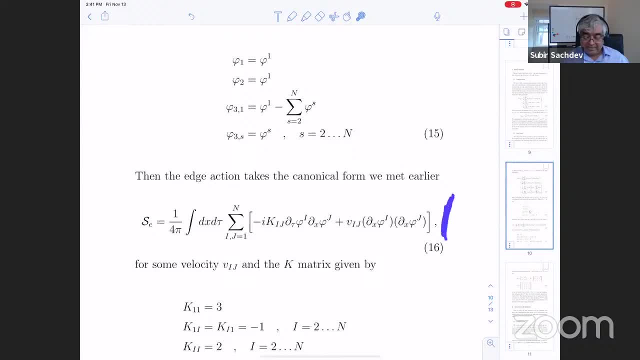 to come up with the final theory, which is this one. This is the theory in the end that survives, which is just fully specified by the K matrix. I see, I see, thank you. There's a question on the chat. Are you allowed to make a part on construction? 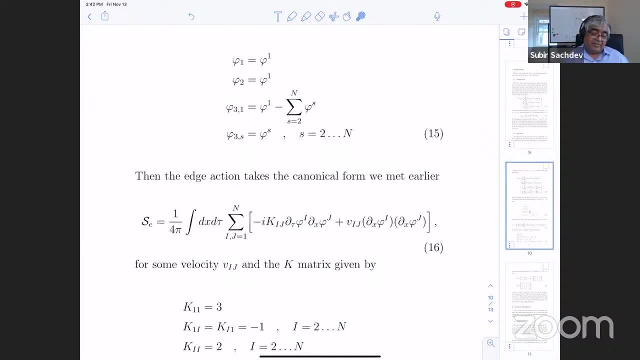 with five partons of electron. seven partons, Yes, you are. In fact, if you wanted to describe the one fifth state, that's the simplest way to do it is to take five partons Once you get to one seventh. 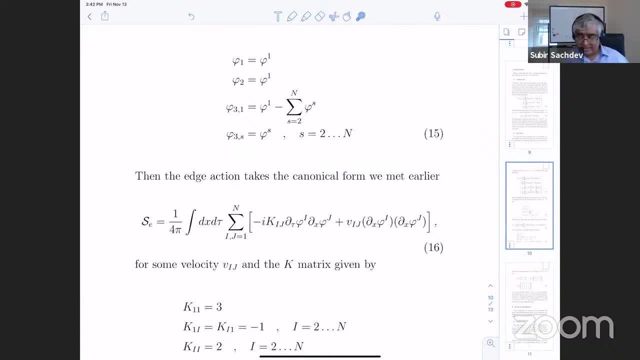 well, the one seventh state doesn't exist because, as far as I know, I think when you get to such low densities of electrons it tends to form a Wigner crystal. One fifth, I think, is observed, but yeah, So generally we don't have to take that many partons. 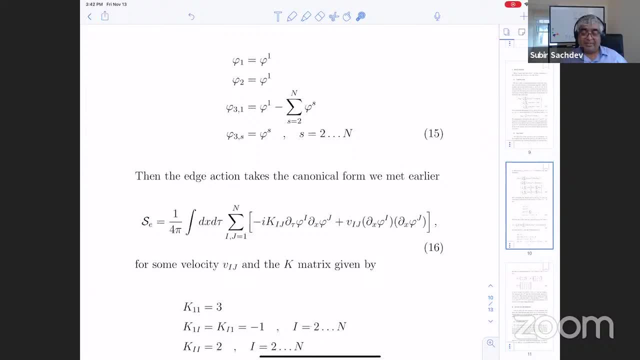 Again, you know, even with the one third state or the one fifth state, you start out with five partons but you end up in the end with just one edge state, because there you have five partons and four constraints. So the partons are, you know, just like the spin-ons. 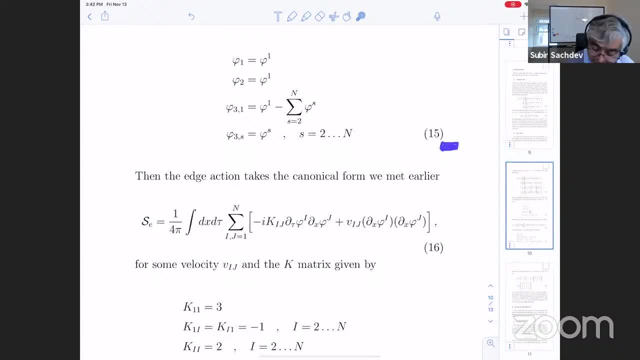 or like the spin-ons, and they're a bit of a theoretical construct, but a very powerful one, because it allows you to, in a very simple way, construct all the gauge invariant information too. Okay, So you know what I've done here, somewhat sneakily. 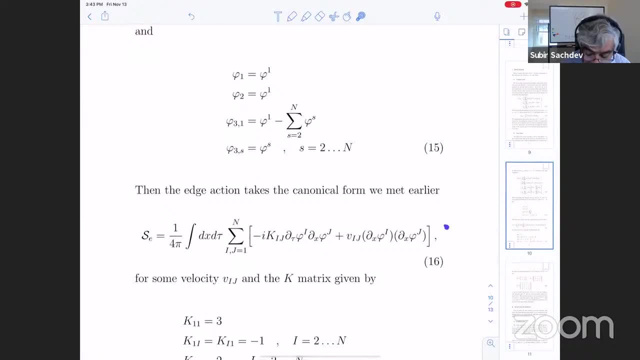 is just done, the edge theory without working on the bulk theory. But you know we learned from our chapter on John Simon's gauge theory that there's a one-to-one correspondence. Once I know the K matrix of the bulk theory, it uniquely fixes, at least for U1 gauge fields. 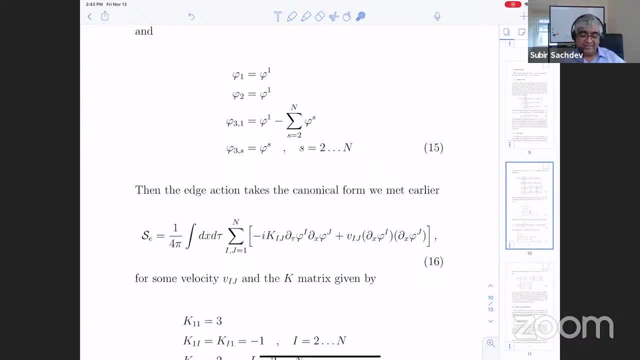 it uniquely fixes the boundary theory, And we fixed it by this somewhat ad hoc argument based upon, you know, fixing the gauge and the boundary and making sure that everything was probably defined in the bulk. Okay, So now we're going to verify that assumption. 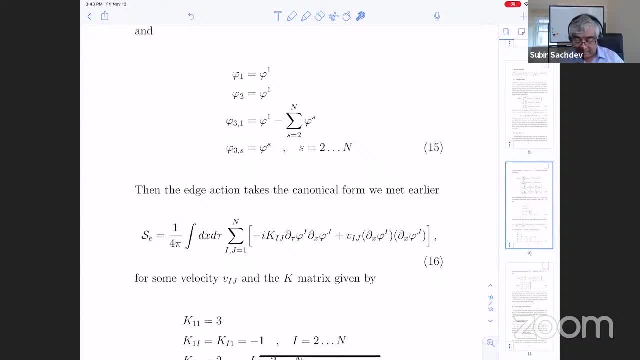 We can now here. we just worked out the edge theory without knowing about the bulk. Now let's just use the same tools to work out the bulk theory. So, for the bulk theory, what do we have to do? Well, we have to just start with this theory here. 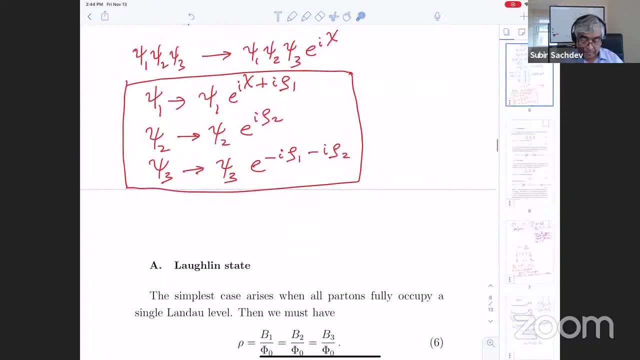 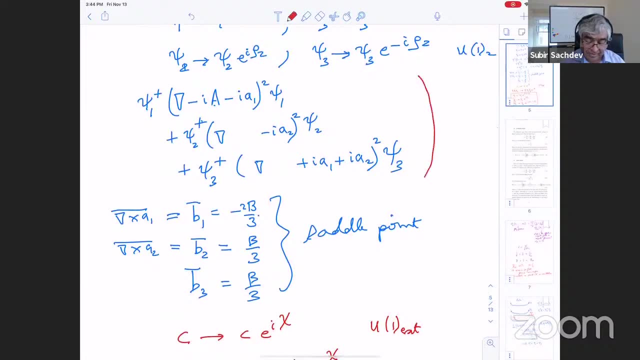 Where was it? Yeah, Yeah, We just start with this theory right here and just integrate out side one, side two, side three. about the saddle point: We have a saddle point. We just again just take the saddle point when the Landau levels. 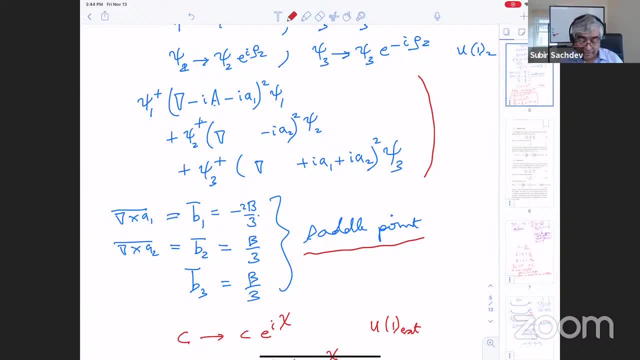 let's just talk about the Laughlin case. So each one of them fully occupies one Landau level. We just integrate it out and you get some effective results. So that's the end of the theory for A1 and A2.. And that should be the end of the story. 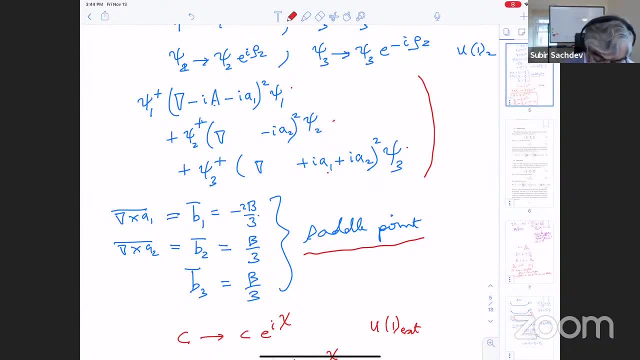 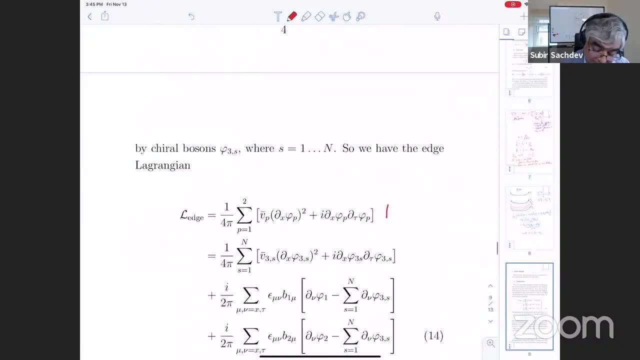 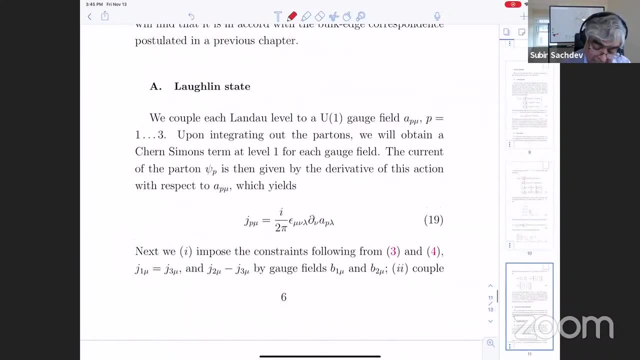 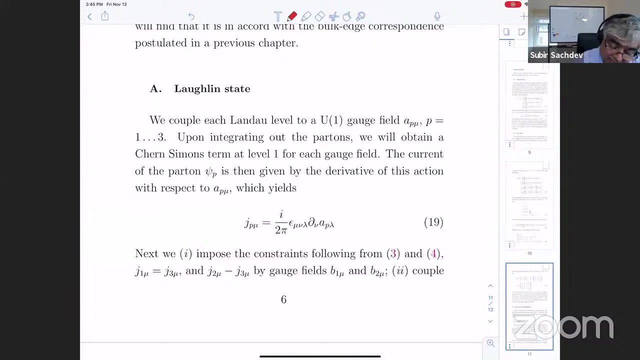 which, for momentarily, we'll just assume, just like we did in the edge, states that that there is an independent gauge field acting on each of the parton. So right now, and unfortunately I apologize for this change of notation, the text, the printed text, is completely consistent. 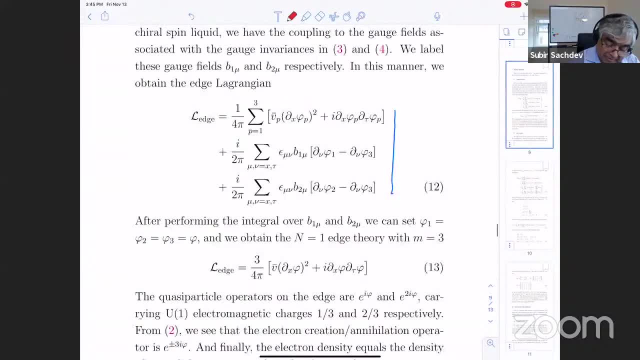 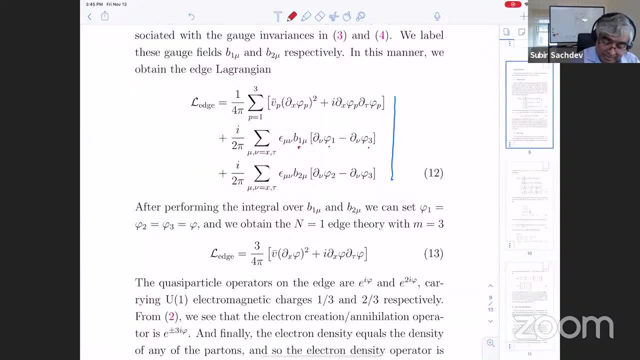 So you know, had for the Laughlin case here a gauge field b1 acting on phi1 and a gauge field minus b1 acting on phi3, and a gauge field b2 acting on phi2, and a gauge field minus b2 acting. 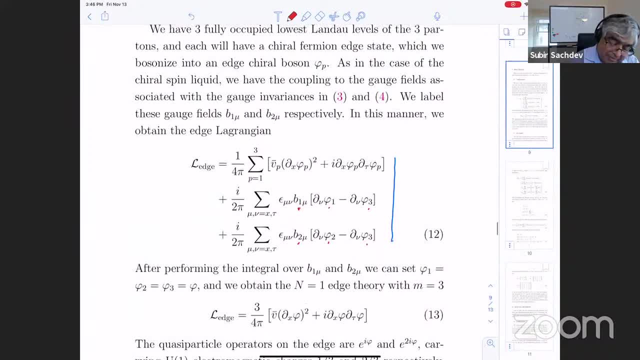 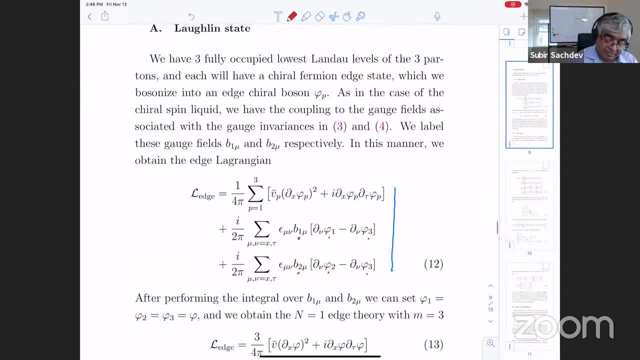 on phi3, or the third particle. So now I'm just going to not think of two gauge fields acting in this way, but I'll take three of them. So basically I'm going to call now. this is where my notation notational faux pas shows. 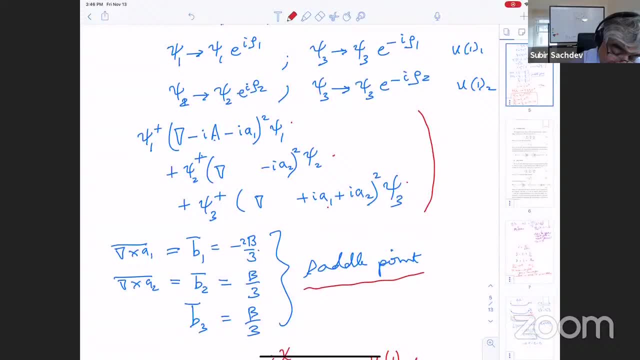 up. so let me fix the notation here, because then it just gets way too confusing. So what I've called is this: oh gosh, this in the notes is called b1, b2, b1, b2, and let's call this capital b1, that's just curl of b1, yeah, actually that's a better notation. 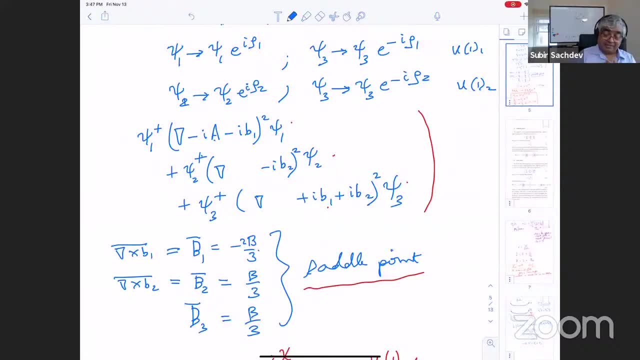 Okay, now I'm going to switch notation on you momentarily and I'm going to call this: whatever the gauge field here, This I'll call a1,, this I'll call a2, and this I'll call a3.. So each parton has a gauge field acting on it, which is ap. so the pth parton and gauge. 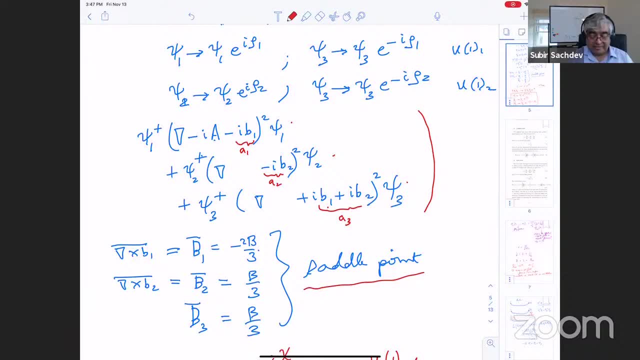 field, ap. Okay then the theory for each one of the partons is just like an integer quantum Hall effect. So we know that we integrate out psi1, all I do is I get a Chern-Simons term for a1, that is the fluctuation about the average field, which is it completely fills in the 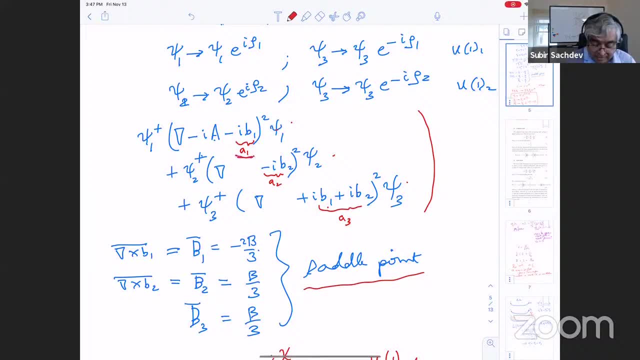 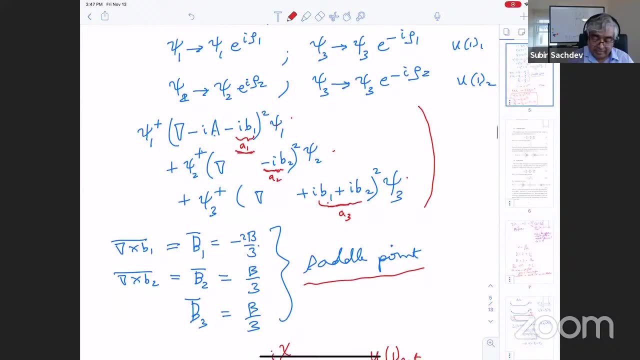 Landau level. So I'm just going to get a Chern-Simons term for a1,, a Chern-Simons term for a2, and a Chern-Simons term for a3 with integer coefficients. This is completely the analog on the edge states. I have these three chiral bosons with 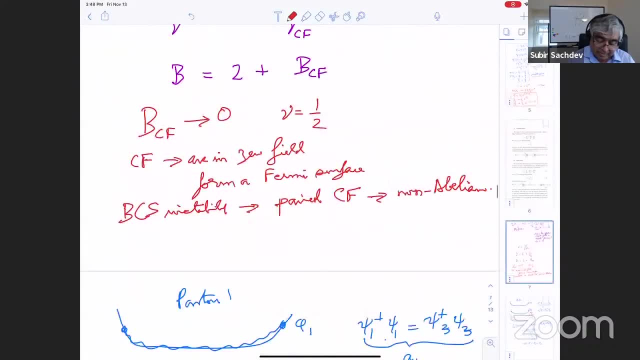 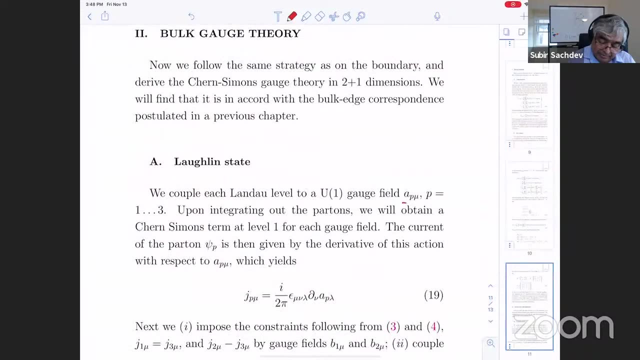 integer coefficients in their action. So basically I'm going to get when I integrate out the bulk, So I have a gauge, Okay. So I have a gauge field ap acting on the pth parton, And then I get a Chern-Simons term which I've written down here for the three partons. 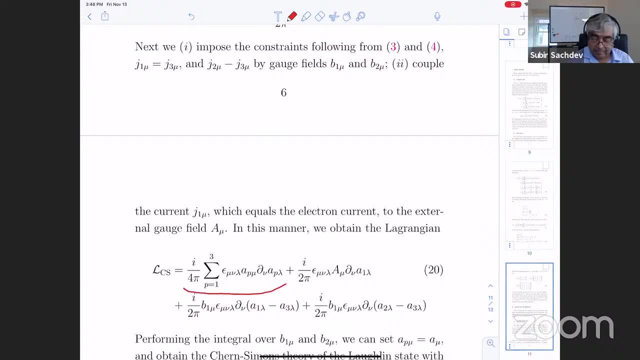 You integrate it out and you get this okay. All right, then. the other useful thing to remember is that I can also express the density on the current of the physical Of the partons in terms of this gauge field, And this is exactly the case that it was for an integer Landau level. 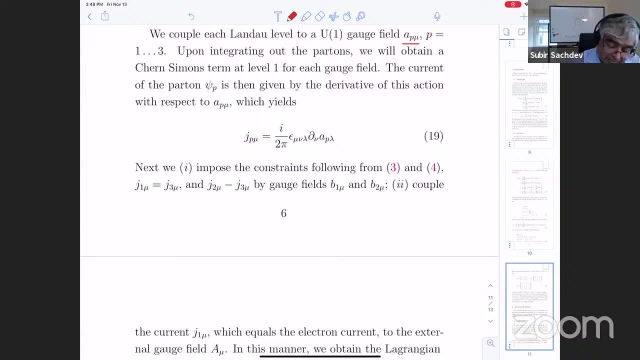 If I had the lowest Landau level filled, then you know we found for electrons that J mu, the electron current. well, the simplest, simplest relation was the following: oops, The basic relation we started with when you have a fully filled Landau level is that 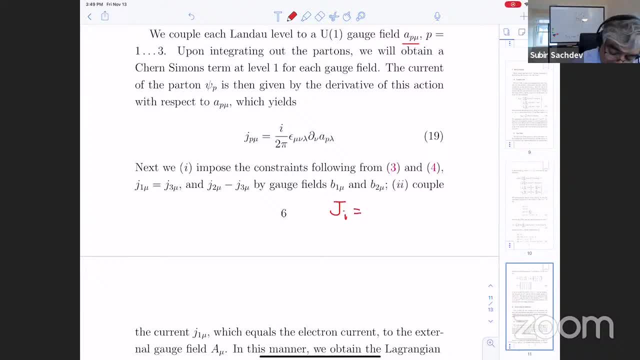 the current J, i Okay, Is the, you know, h over e squared here is basically the hall conductivity times the electric field And this is, you know, integer, in this case, basically one times epsilon, ij times ej, And you can now by gauge invariance. you can write the: well, there was a two pi the. 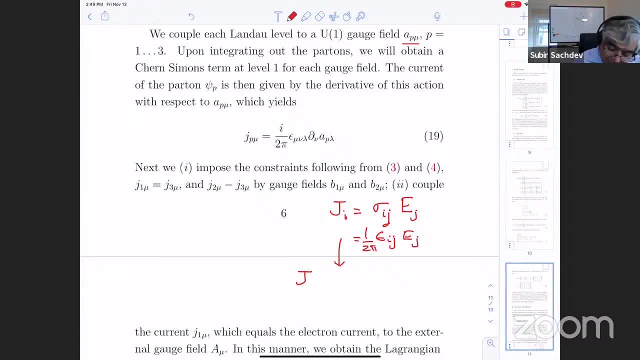 one is a one over two pi for integer Landau level. So the relativistic generalization of it, or the really the gauging variance generalization, is epsilon mu nu lambda. The new a lambda is what's the external field, So here this, the internal field that's acting. 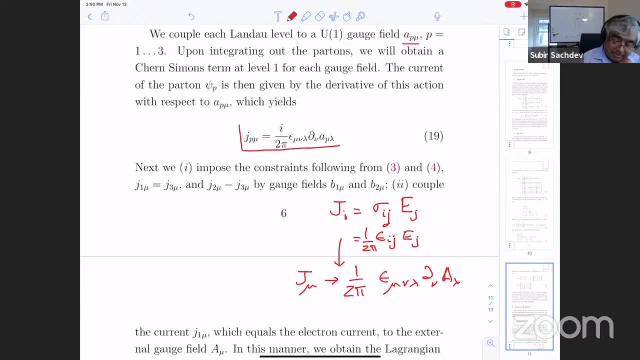 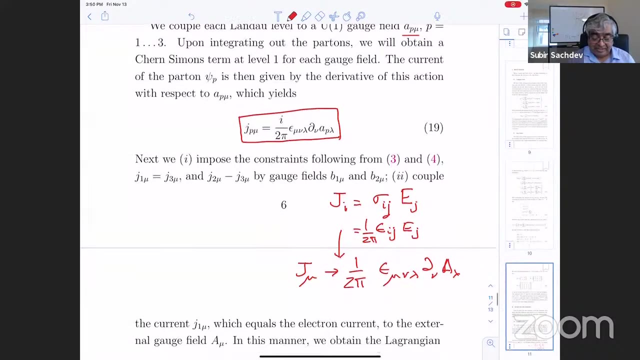 So therefore, for each part on the current of the parton, it's just the curl of the- because you're in a exactly an integer filled Landau level is just the curl of the internal gauge field. Okay, so therefore, now I'm almost home free. 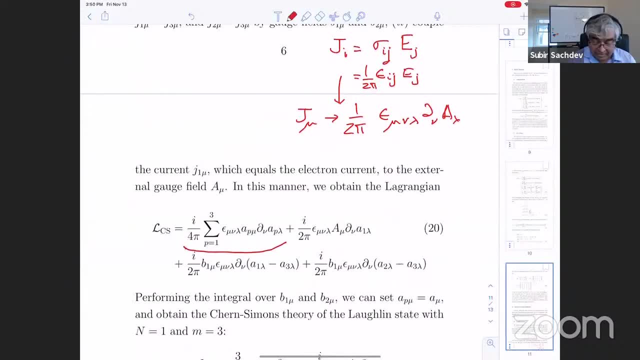 I integrate out the electrons, the partons, sorry, and I get a Chen-Simons term for each of them. Then I couple the external magnetic field to the current of each of the partons, but the current is this, In fact, only the first parton, sorry. 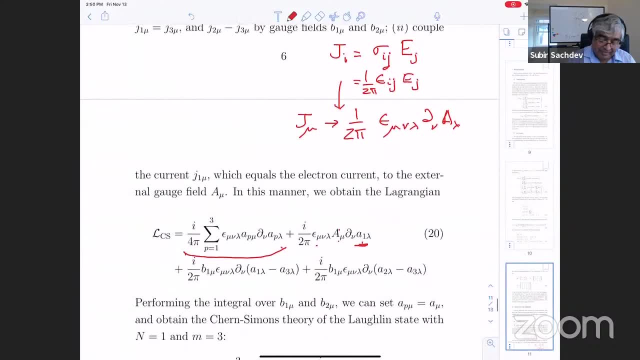 the external field only couples to the first parton, And then I have a constraint. The constraint is that the current of the first parton equals the current of the third parton, And that's exactly this. This is exposed, implemented by another Lagrange multiplier. 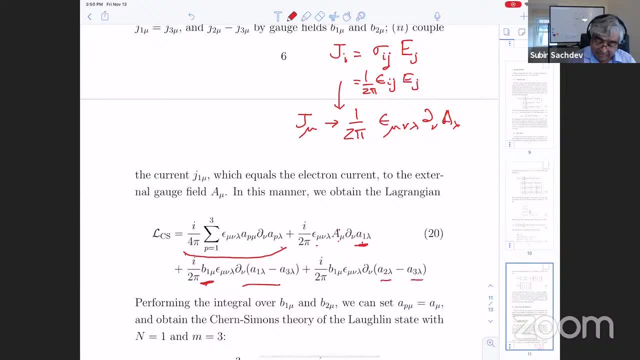 And then the current of the second parton equals the current of the third parton, And that should be a two over there. This is day two, mu okay, And now I'm pretty much done And now I can integrate over B1. 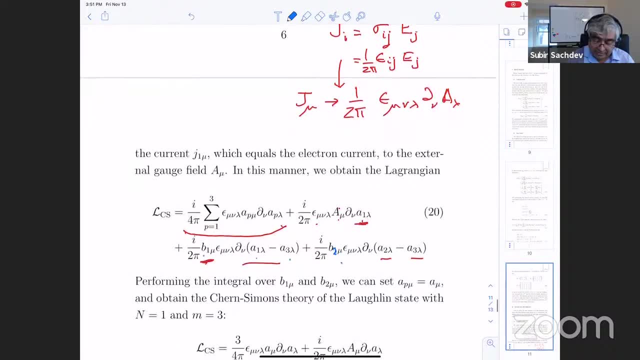 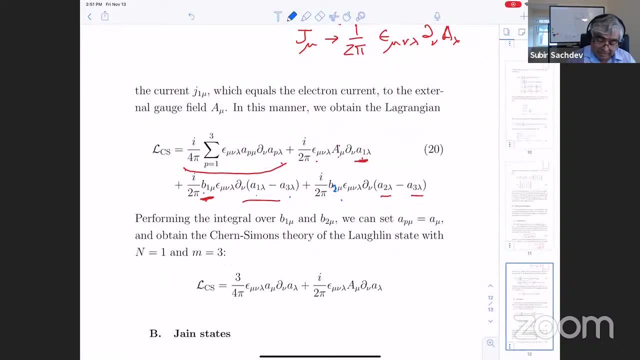 and B2, I get a Delta function of the three gauge fields and I'm left with just one gauge field. And then I also have this becomes and just call it a mu, And there's my Chen-Simons gauge theory for the Laughlin state. 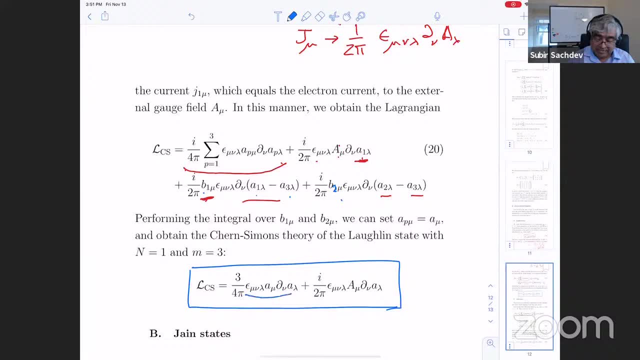 You have the Chen-Simons term at level three for the emergent gauge field, a mu. There's only one emergent gauge field. after you impose the constraint And the part runs And then and the external electromagnetic field couples to the flux of the internal gauge field. 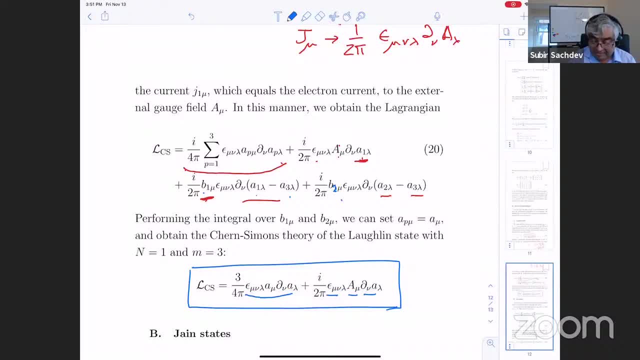 And this is the same as coupling to the elect, you know, to the, to the physical charges, because each flux is tied to a charge by this relation associated with the Hall conductivity. So you know this, this thing, there's nothing but a mu the mu. 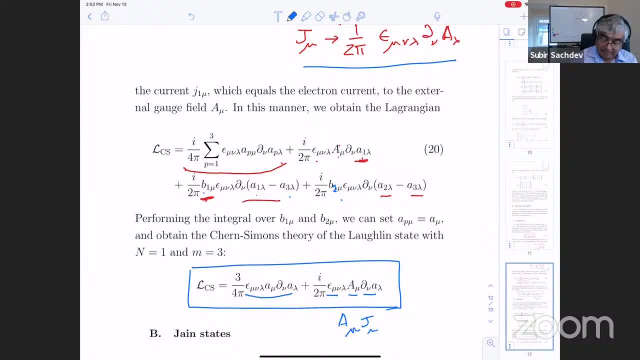 which is the usual coupling between between the electromagnetic field and the current. But here we've written the current in terms of the emergent gauge field, little a. Okay, So yeah, so that's the famous result of Chen-Simons theory of a Laughlin state. 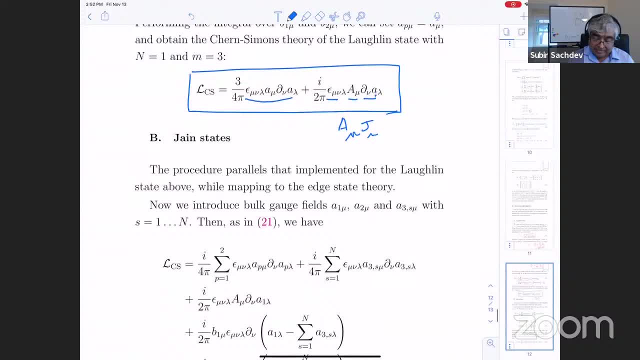 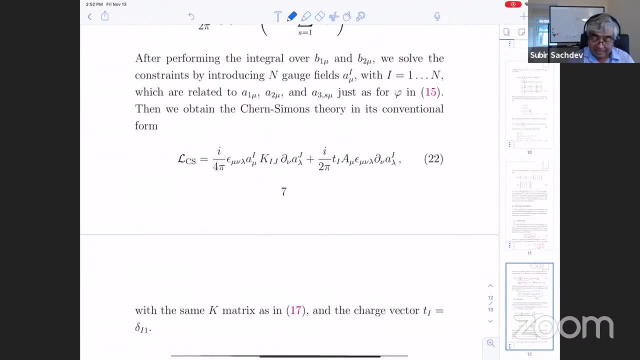 And the Jain state. really, you know it's, it's. you know, I don't need to say more. You just turn the same crank and you get. you know exactly what you would have expected. You get the same K matrix as you found in the edge state. 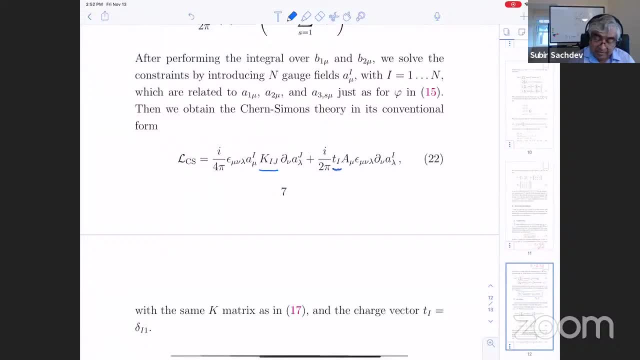 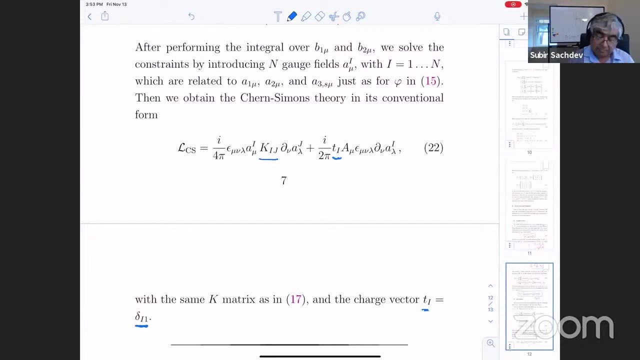 And now you have this T vector telling you what does the gauge field, which of the internal gauge fields does it couple to? And it basically only couples to the first one: delta I1.. That's the T, this T vector. Okay, 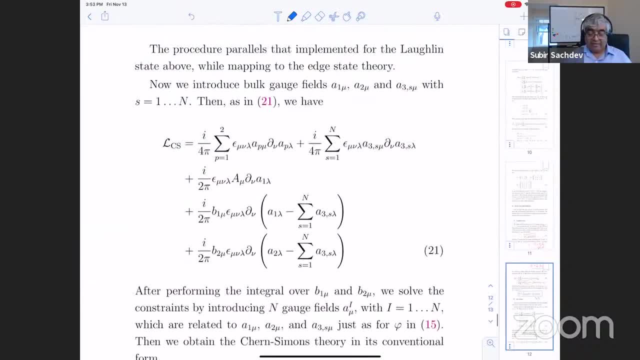 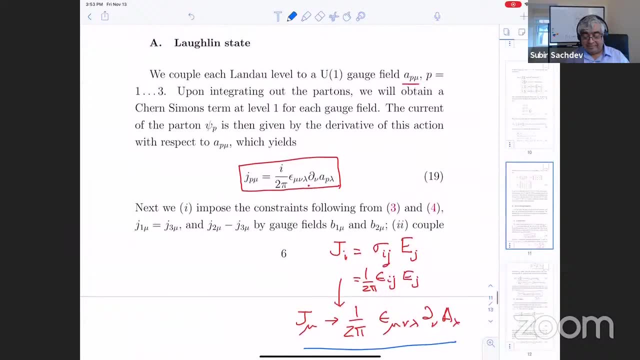 All right, I think that's all I have to say about the fractional quantum Hall effect. You know that was very rapid, I admit. Probably covered about 10 years of history there, but hopefully, with all this tough preparatory work we did in this course for the past month or two, 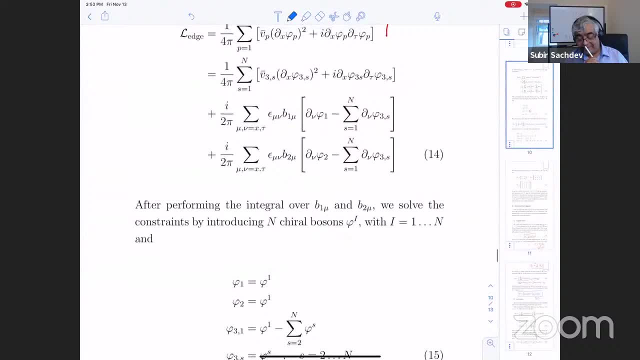 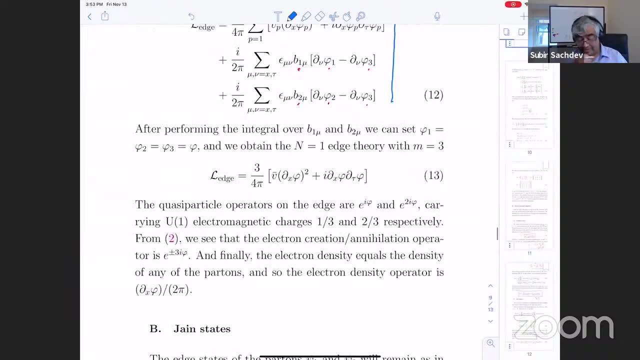 I'm sure we'll be able to get to the next one. So thank you very much for your attention And I'll see you in the next one. Bye-bye. You can see how it all looks- totally obvious, I hope by now. 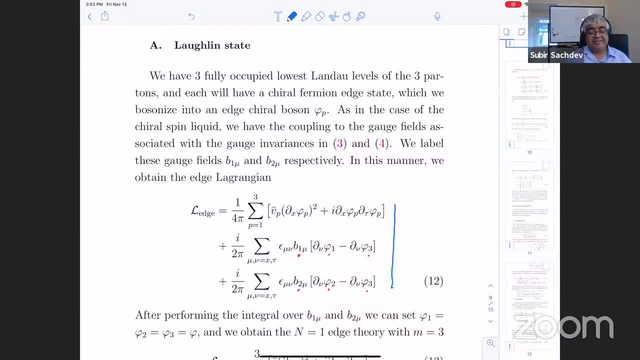 Of course, it wasn't obvious by the people who discovered all this. It took a while, But once you present it this way, it almost seems like all you're doing is turning the crank. but that's because I prepared you with the right sort of 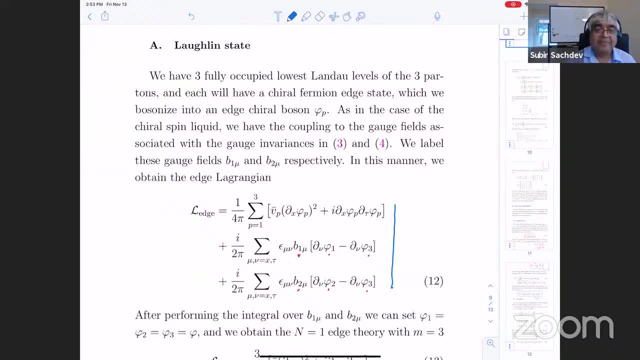 tool to turn these cranks. Okay, so the question is: n1 equals 1, n2 equals n3 equals 2.. It seems like you have nu equals 1, 1⁄2.. I don't believe you do. 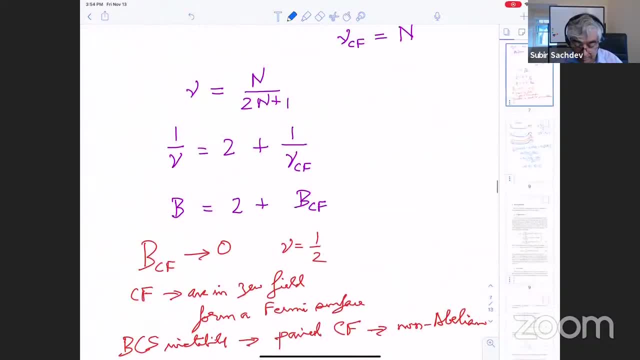 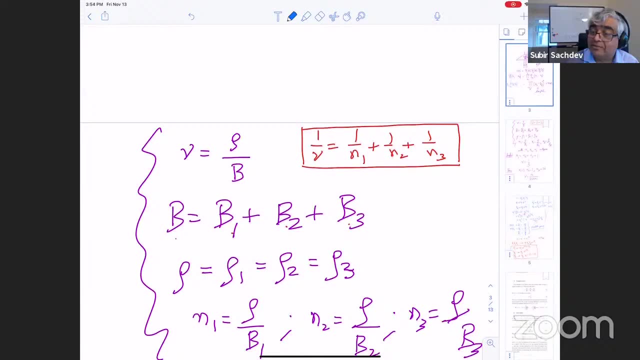 So if you put it in here, let's just work it out. So what you say for n1 equals 1, n2 equals n3 equals 2. So then 1 over nu is 1 plus 1 1⁄2 plus 1 1⁄2. 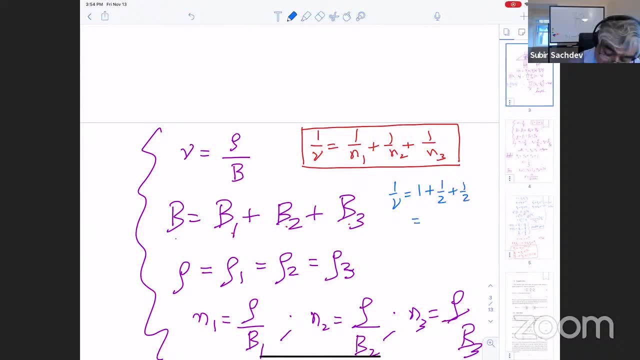 Plus 1 1⁄2, which gives you 2,. wait a second, all right, What did I do? There must be some constraints on n1 and n2 and n3, okay, What's going on here? Somebody rescued me. 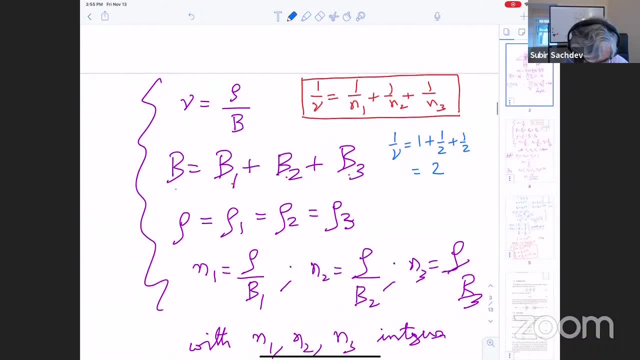 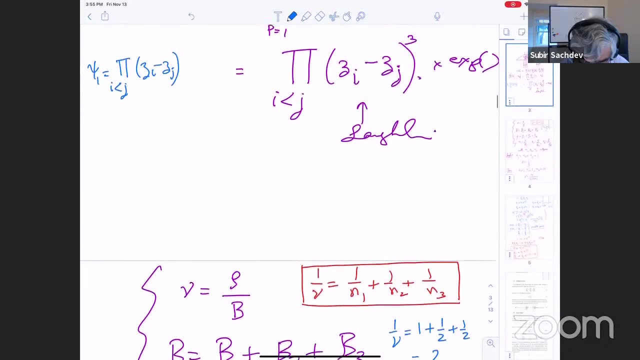 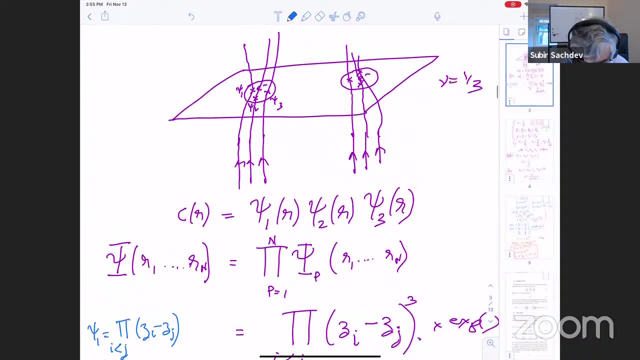 Good question. Why is that? And that gives you nu equals 1 1⁄2.. That doesn't make any sense. Let's see. Is the fermionic part making sense here? Is it just because the setup point here is not stable? 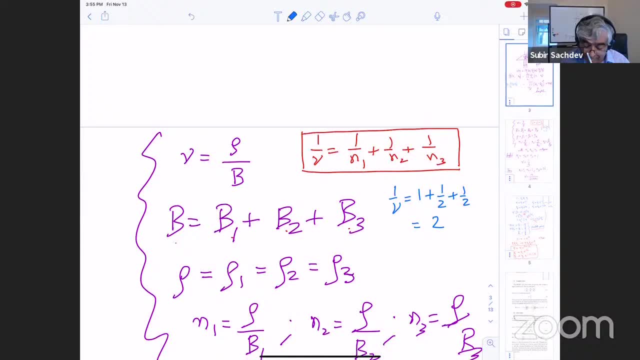 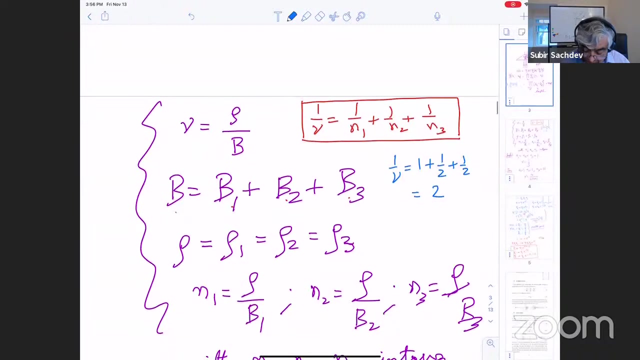 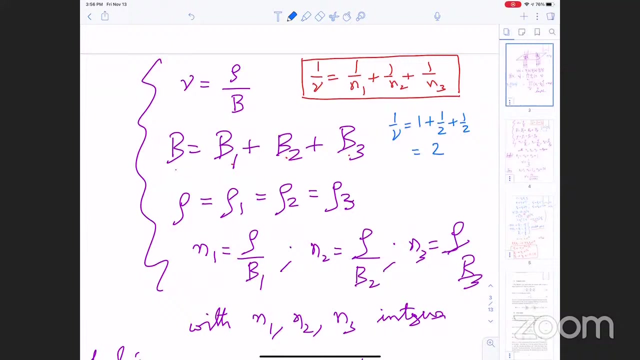 That could be an answer. I'm just a little worried that somehow I've forgotten some important point about the whole wave function being anti-symmetric somewhere, because these have to be fermions. Did I do this right? Okay, Okay, Yeah, but since each 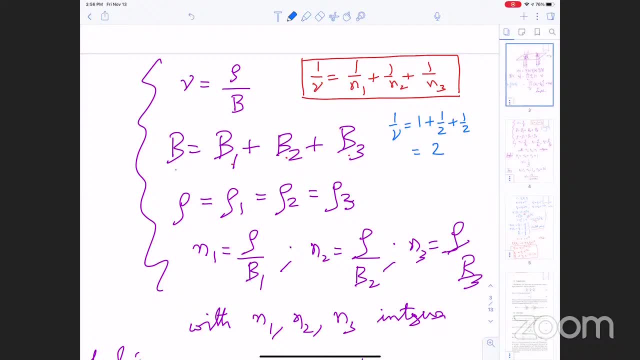 each part of the wave function is anti-symmetric. then you take a product of three of them. it should be symmetric, right? It should be anti-symmetric, Yeah, So that's okay. Okay, I mean, maybe that is a possible state. 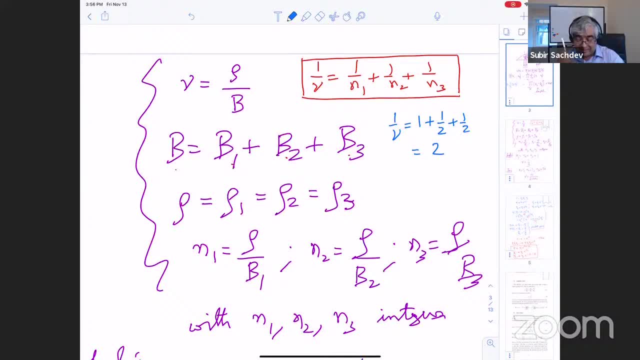 nu equals 1⁄2,, but it's not the one that's observed. That I'm pretty sure. So that's an interesting state And yeah, I guess, maybe. okay, I'm guessing, maybe I've made some conceptual error here. 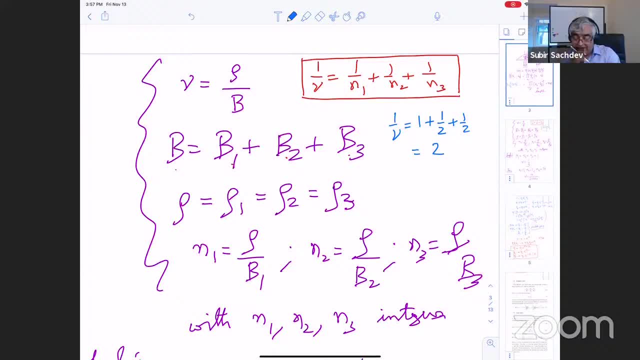 I have to double check. I'll think about it over the weekend, But my guess is that so far it seems like, yeah, you're right, You could get one high nu equals 1⁄2, but that's not the nu equals 1⁄2 state. 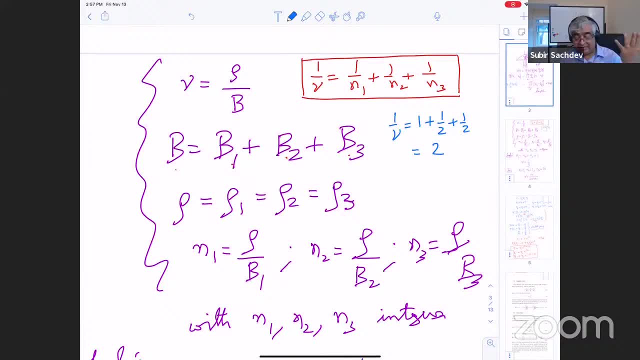 that's seen in experiments. I mean, this kind of procedure just gives you some states without giving you any idea of why the energy is good. Whether there are good variational wave functions, probably they're not. this one is not. So to be animal-like here. 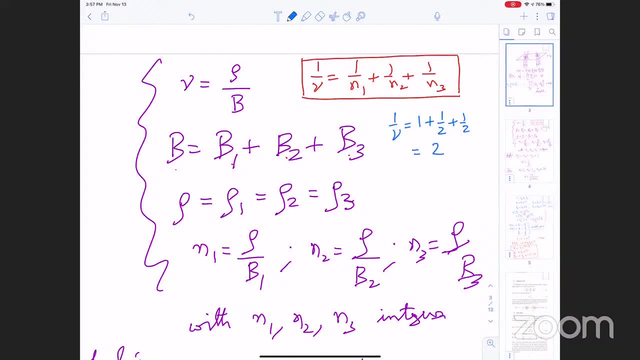 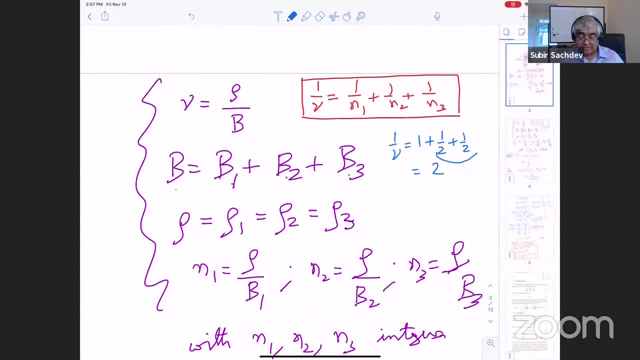 you might need to consider the SU symmetry. Yeah, I was thinking about that too, right? I mean, if you put two of them in this second Landau level, then you should at least at least do an SU with respect to the two of them. 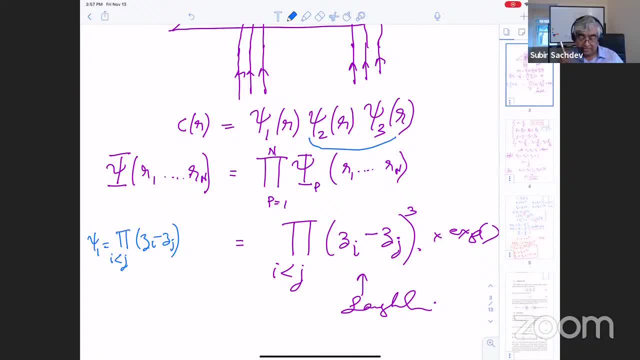 And we have to worry about that, and that might make that whole thing not not well defined. There may be some subtlety in the structure of the gauge fluctuations. It's possible, Okay, well, that's a great question. I'm sorry I don't have. I have an answer, but I'm not. 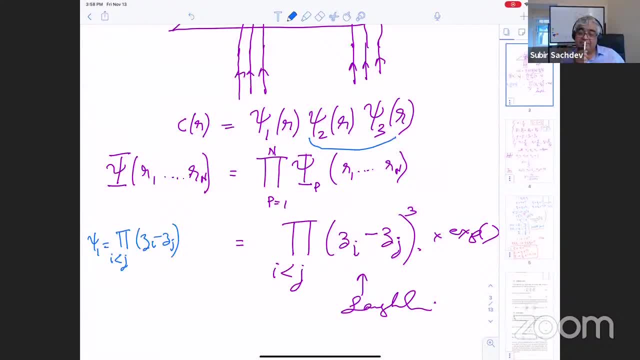 totally convinced that I gave you the right answer. Yeah, I'll ask some of my colleagues who are more experts at fashion quantum hall than I am, Or maybe you can ask and let us know on Monday. Okay, I don't have more to say here.